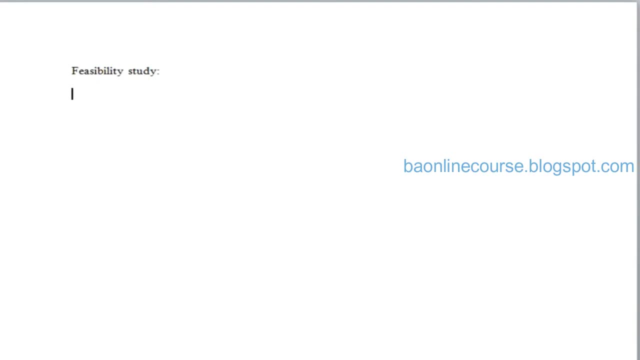 construct a dam. they want to construct a dam. why they want to construct? because they want to construct a dam to streamline the water resources to the paddy fields, so that the paddy fields will grow properly, so that farmers will be happy. so this, for that reason, usually make irrigation projects and because of 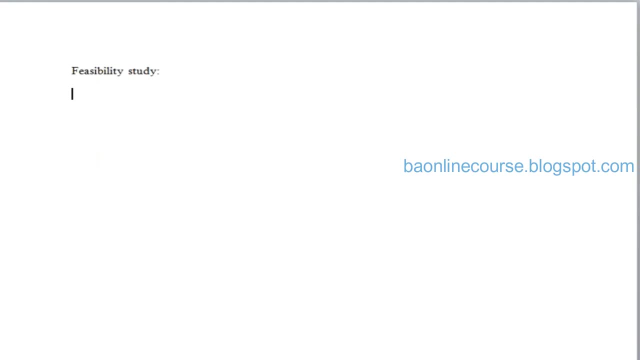 this reason irrigation projects will not occur. so when we were constructing some irrigation projects and all that generally which was taken care before government has taken a decision of constructing some irrigation projects and before they are calling for some qualified construction companies to construct that pad before itself, they do a feasibility. 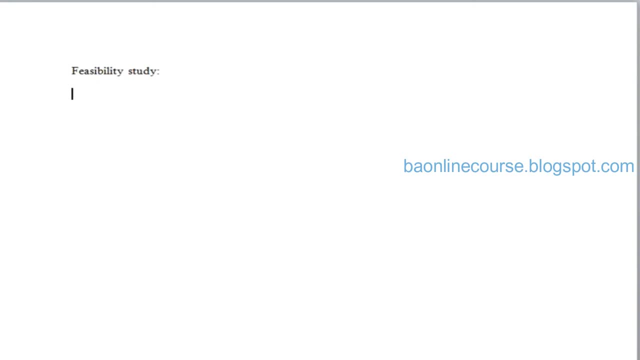 report. the arrangement is usually for management consultants in between, whatever the decision government has taken, and all will be informed to the management consultants. so these management consultants were experienced, right. so these are all the experienced professionals who are involved in the management consultancy. so these management consultants were experienced, right. so these are all the experienced. 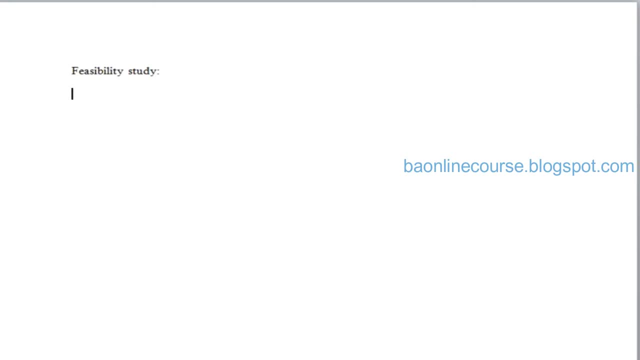 professionals in the irrigation project construction and all that. so they submit the feasibility study report and the government will ask these consultants to provide a feasibility study report. what is meant by a feasibility study report? feasibility study report doesn't mean the area where they want to construct. okay, where it has to be constructed in the 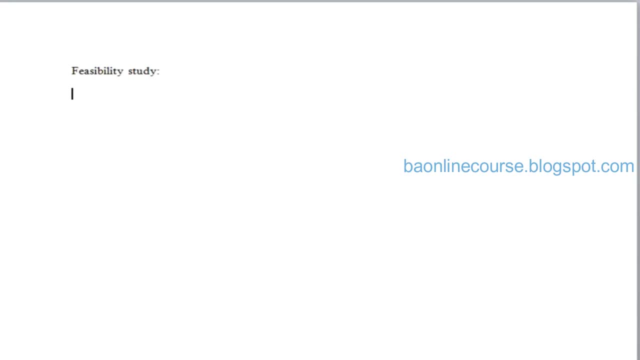 place need to be identified in the canine, because water man irrigation projects like to get a pool deprecation risk. dedication for project general dam, low water dehydration, that image talk JC. whenever the water is required enough, damn gates simply indicates the mood gates after that so that water is required. that if the gate is 2 gates or 3 gates, then so that is how thiscasly possible to construct a dam irrigation project. at which place? then a two gates or three gates to construct a dam irrigation project in this cas will not work. the biggest ten for this anywhere because, yeah, you will produce in general cas, relax work and if you 할 acit, activity will still be instance. water must be there if the atmosphere is less so in this factors, if it has no. 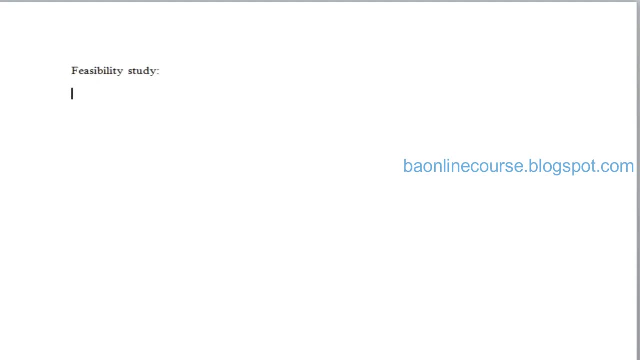 then Tulsiq would not let us do so- that water flow will go and then in the lower levels, where there are fields, water will go to those fields. This is water management. This is what is generally done. So you can construct a dam anywhere you want. 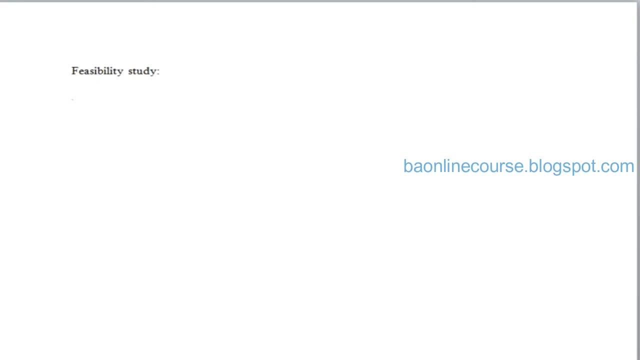 For example, if the government has identified a place to construct, they can construct. So why should a management consultant tell you- Because the government is an authorized person to do that- What change They have all So they can immediately. they can call for the qualified construction companies to start that. 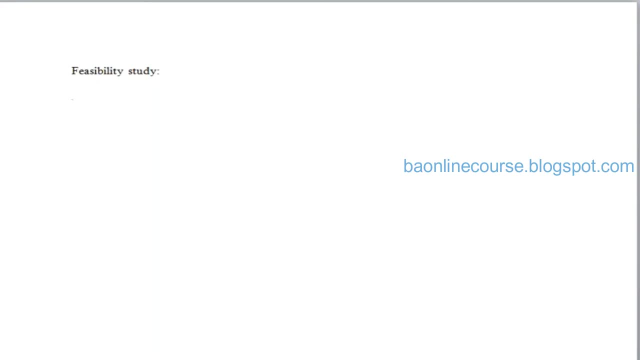 So in Bheechme, meanwhile, why they require a management consultant to provide a feasibility study report? Why is it needed? Any reason? Why is this required? Any idea To check whether everything is in place for the management. In place means In terms of 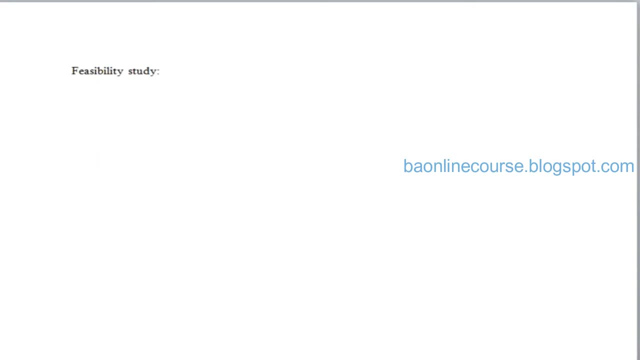 In terms of all the aspects, like you know, water management and like you know building-wise, everything Right, building-wise, Building-wise doesn't mean So. the soil should have a nature, should not have a nature of sinking. 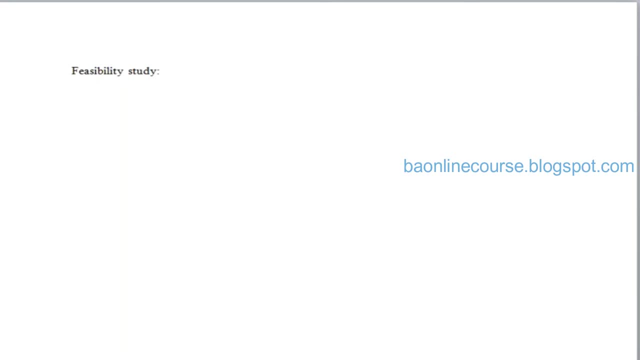 If the soil has a sinking nature, Irrigation project construction Is it required? Is it required Custom Why Sinking nature is in place for a period of time? Dam will be in the problem, Isn't it Right? That means soil testing is done. 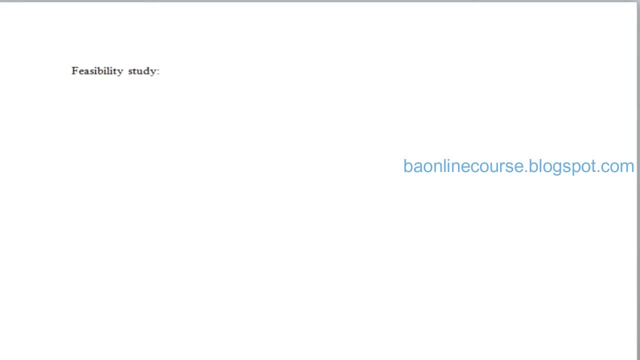 That means, is it required for us to build a dam here? If we construct a dam in any place, if we construct an irrigation project, it is an advantage for us. If we build an irrigation project in any area, it is an advantage for us. 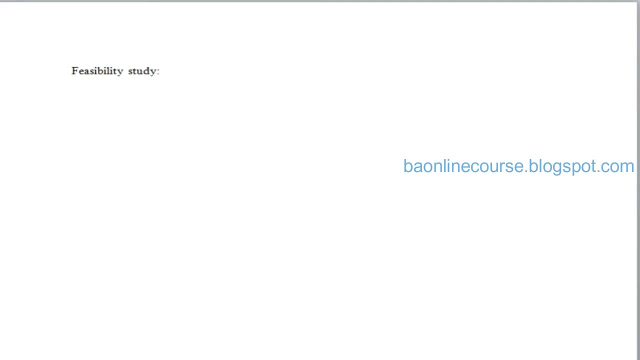 Right Any place we construct soil testing in that area. all these are the responsibility of management consultants. What they do is they will prepare a feasibility study report And they will submit it to the government. That means before the government takes a proposal. after taking a proposal, they call for feasibility study report for confirmation. 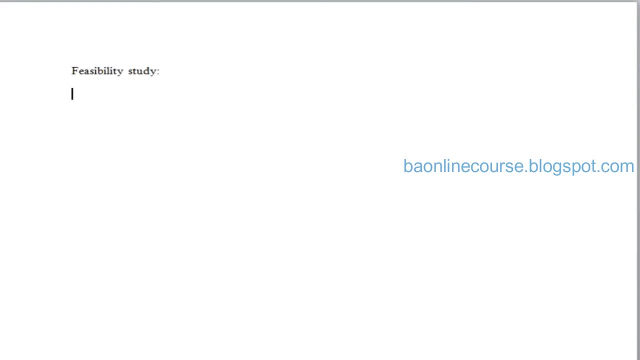 What these consultants do is they do ground soil testing and so on. Next area: Where do you want to go? What is the cost for that? These budgets, All these are generally done by them. After that, what the government does is: the government will call for the tender. 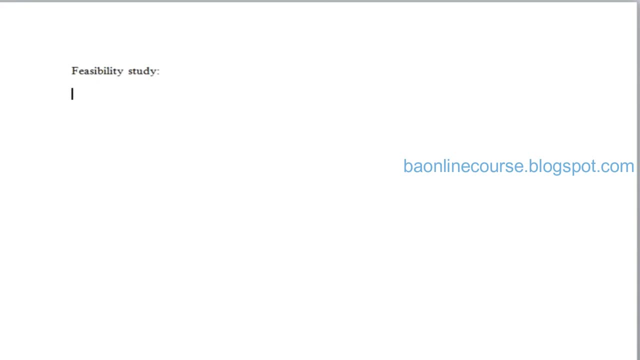 For the companies to come and bid based on the conditions, what has been mentioned so far. What is happening here is when we want to take up some decision of constructing something, we were working on feasibility- What is feasibility? Soil testing should be done. 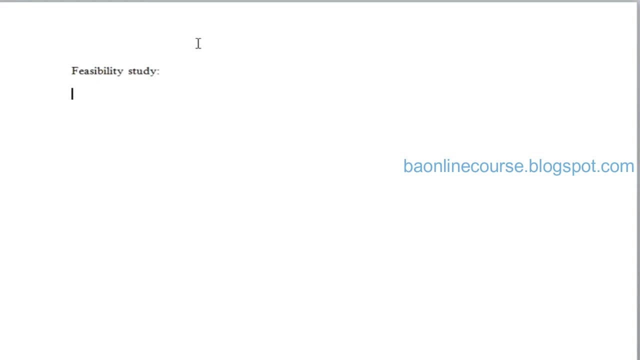 Why should it be done? Because the dam construction should be done properly. It should not be sinking Point number one, Point number two, Wherever we are constructing the place to be constructed, not only now but in future. it should be useful. 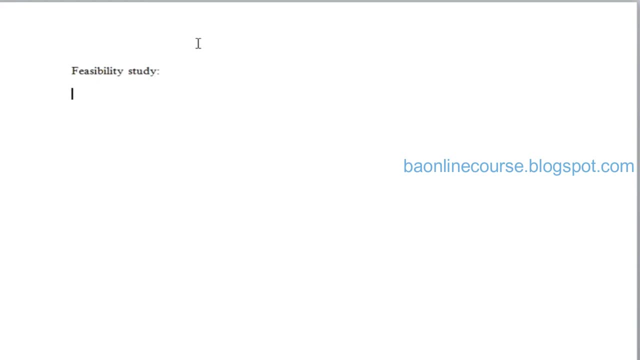 For the farmers around us. it should be useful for lakhs of hectares of land. Point number three: Because of that, another sinking village, Sinking villages. We call it Mumbu Grama in Telugu. Because of that, in any village there are chances of sinking in the surrounding villages. 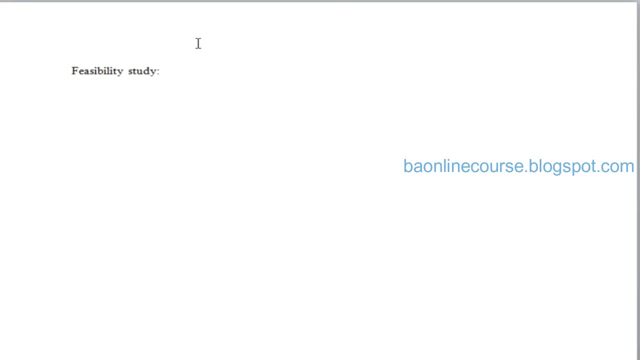 What should we do about that? We took the survey report and evacuated them to another place. We brought them to the construction site. So all these are ground reality. To make a decision in the boardroom, ground reality means the reality you took on the ground. 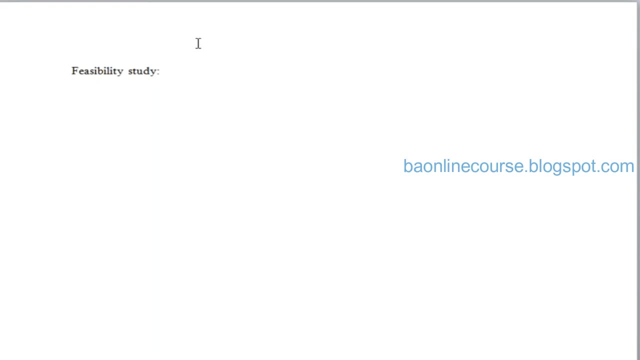 What is the difference between the reality you took on the ground and the reality you took on the ground? Is it so In the boardroom, there should be variations between the decisions you took on the ground. Why is that? Because they personally see everything that is going on. 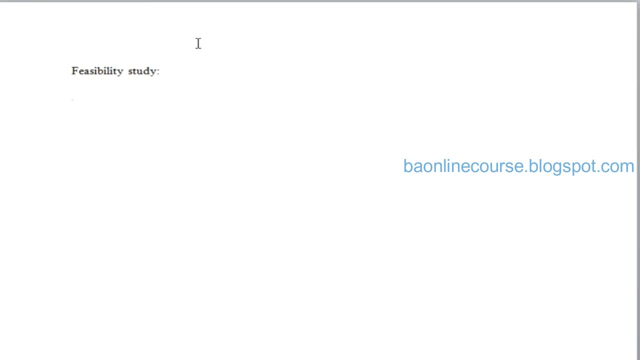 Absolutely What is going on Where we have to construct, How it is to be constructed, What will be the budget Right, How big this irrigation project should be And how many lakhs of hectares should be built, of hectares should be fertile because of this, and what will be the benefit for the farmers and all. 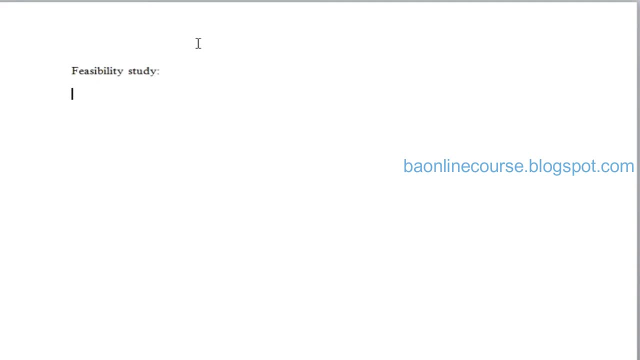 in what way? okay, water, i can't just in finding just in the water. and happy can the company's not at the given age of art. and happy, lift irrigation. the outer side is strong. it's a. it's not a human made together. it's a, it's a nature, it's nature, it's a nature made. so on the atlanta. 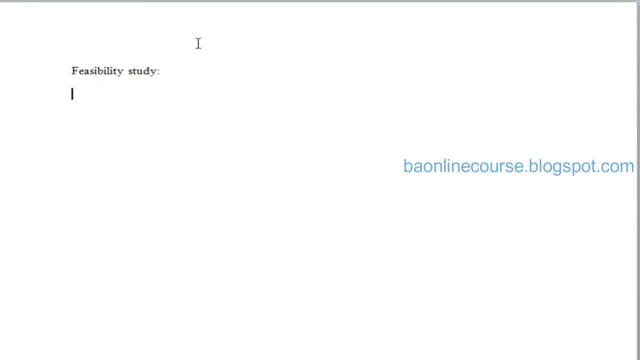 which, but end of the dangerly water pollen. only up can make water. so a feasibility study report a government has taken together when they want to construct something or when someone some. when government has decided to submit a online video meeting pro bidding is in the paper a little bit, this window. 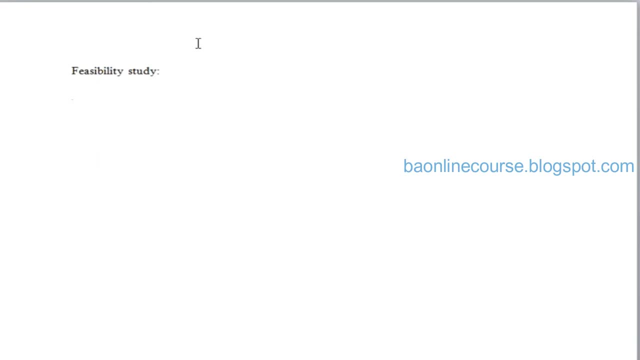 what is the government is? the government has taken it, it's taking a decision of, it's taking a decision of a feasibility study report. okay, please, please, study report, please, ability study report basis. in the same way, when we were developing some project, project management management, for example. 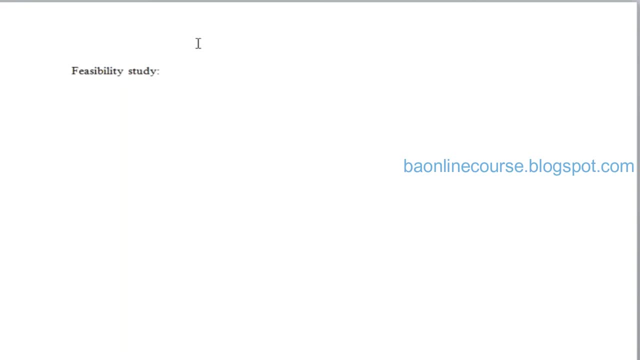 man it projects, financial healthcare projects. when we want to construct a plan, when we want to construct any of the place right, any of the, any of the project and all, when we want to build any of the projects, we have to see the feasibility. you can feasibility in two times. 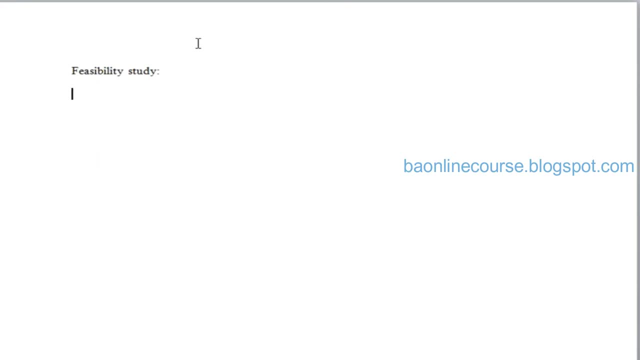 feasibility. an employee will see and the client will see feasibility. we also will see a feasibility employee in the future. at the same time, why are we doing this? what is the feasibility for us to do it and all and then? so two type of feasibility, isn't it and the project project? 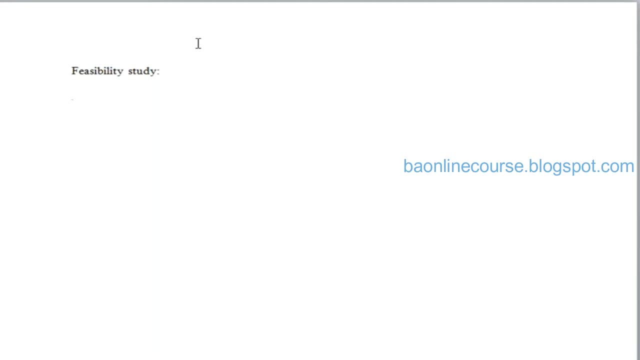 is because it should be useful for their professional growth. yeah, understood, company group doesn't mean company growth i'm talking about. so this feasibility study report usually divided in three parts: vocative technical. next operational, next financial, financial feasibility. so these are the three major feasibilities which are there for any of the project to be done, this feasibility study. 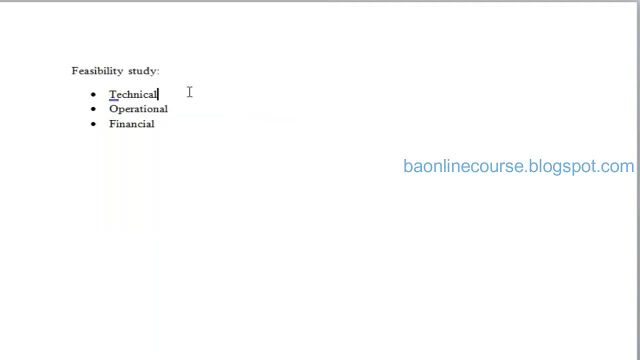 report should also be done by us. so one is about technical feasibility, technical feasibility and to come to study about the technical feasibility, we have to study about the existing system in the market. existing system. what kind of hardware and software infrastructure the client has proposed system? no water, all need to be developed features. 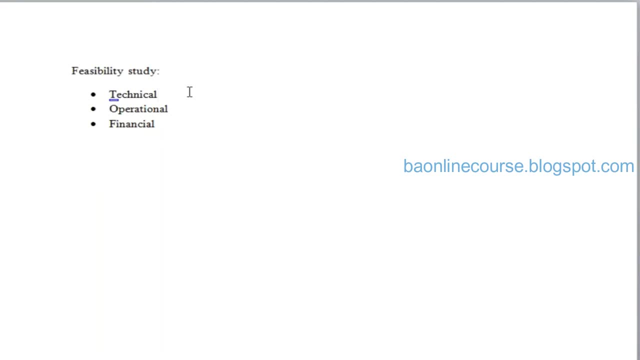 knowledge to have been developed and all. is this compatible with the existing hardware and software infrastructure or anything to be updated? okay, this. he is asking for us about more security features and all that, but the basically, if the existing application intend to have a basic legacy application, okay, world systems online, usually. so what an update. this is what we call it as. 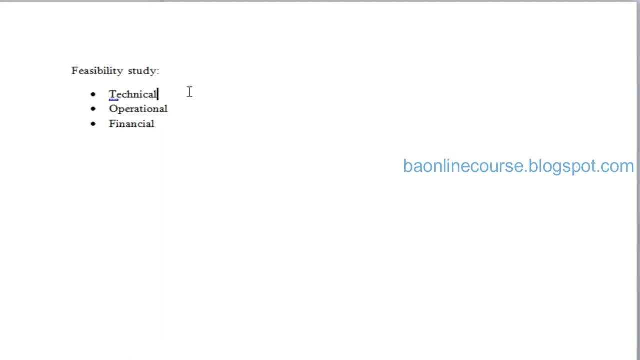 technical feasibility. this we call it as technical feasibility, technical guy and feasible. we have to look for our own clarification now we have to take our own clarification whether how far is this will work out. again, decision this call, so the kind of feasibility, what we do call it as. 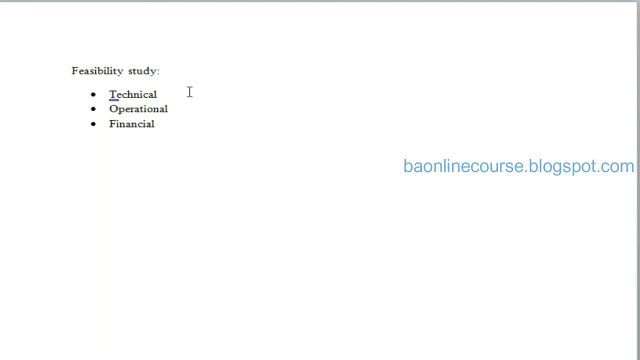 technical feasibility, we call it as operational feasibility. what is meant by an operational feasibility? operational feasibility doesn't mean not only of developing the project. at the same time the project should able in a position to used by the people until an application developed. jason economy water code and copy of the new in the new project, this code on the regular. 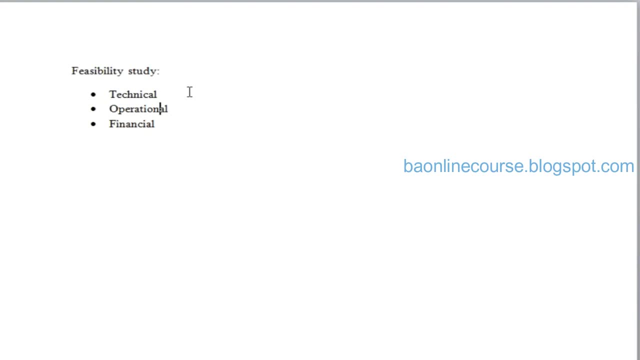 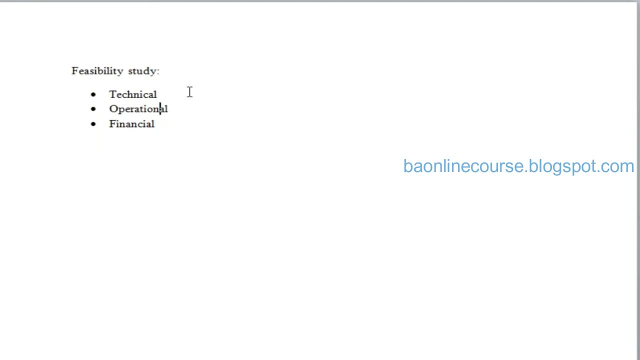 and day and day. it should be compatible for a client to use it. it should be compatible for a client to use it. it should be compatible for a client to use it and it should not be so complex another and it should not be so complex another and it should not be so complex another. yeah, it should not be so complex. 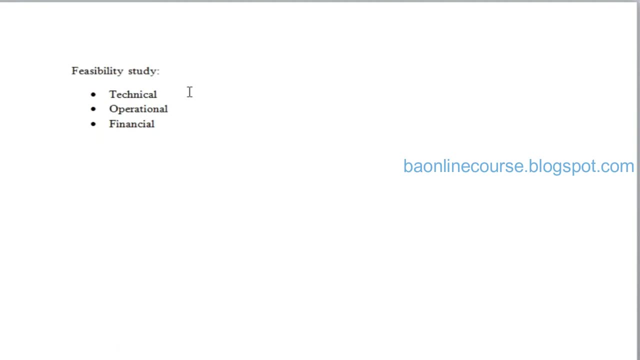 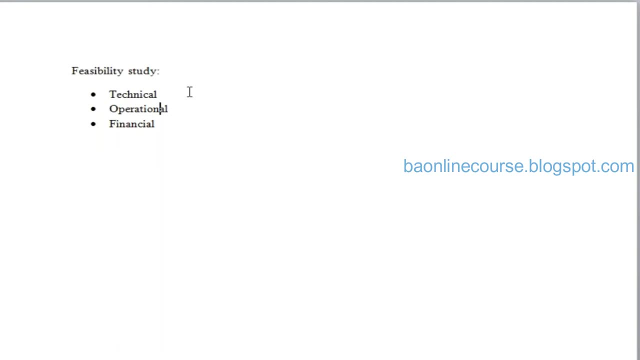 it should be user friendly. this is what we call it as operational feasibility. operational feasibility- operational feasibility- understand, yeah? third, we call it as financial feasibility. financial feasibility, which means what is the cost we have taken and all the money calculated, and a financial feasibility. so feasibility study report will be of three types. when we call it as a, 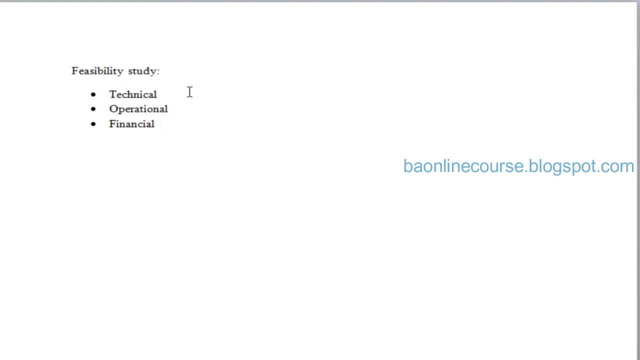 technical feasibility. second, we call it as operational feasibility. third, we call it as financial feasibility. this feasibility study report, or feasibility study, should also be done in the initial stages of the project: clear, clear him and then yes, yes, yeah. so once the feasibility study report is completed, then do we do for stakeholder analysis? we do for stakeholder analysis. what is? meant by stakeholder analysis? what is it required? how is it required? so feasibility study, a stakeholder analysis, and taking stakeholders analysis doesn't mean people who, over directly or indirectly involved in the project, will be called as a stakeholders or clients. go to lay the technical developers, go to testers, go to project manager, go to solution architects, go to. 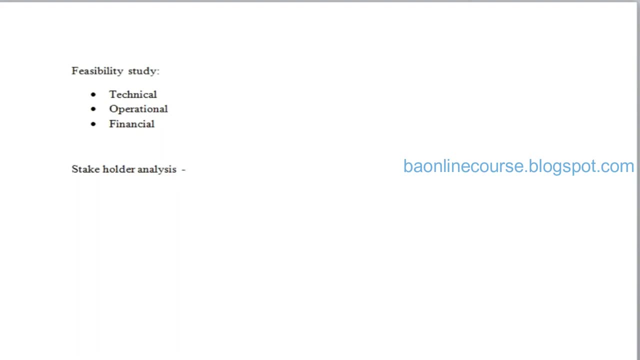 read about. you know the minimum amount of stakeholders will be called as stakeholders going to test like that. why you want to test, focus on, you know, on technology. why will you be? you know a tornado or nuclear contained at you are not involved. this is clearly a long story and we can get into this decline and wonders due. 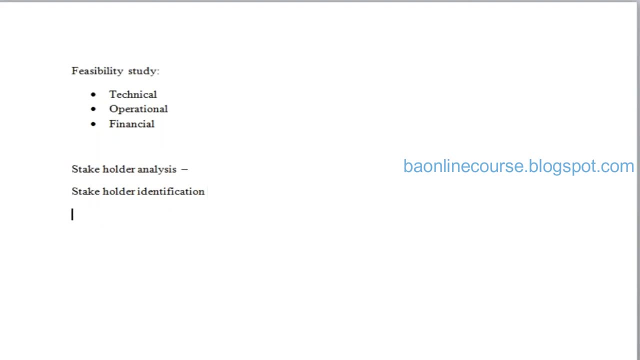 to the direct feed early interaction. we find it gradually the system takes away in different phases of the process through. You can tell me, as I said specifically in a different critical people, unless there is a technical failure which has say okay, a predictor to better reason, either you change that or's not going to. happen or if you find you will need a different system. basically, the teaching paper will take the testers from two very specific paths, always to HIS teachers, because they are hidden from the researchers at at that time. you'll and Stormy, he says that. how can forget. pretty much, did not? they have credit as leverage of the 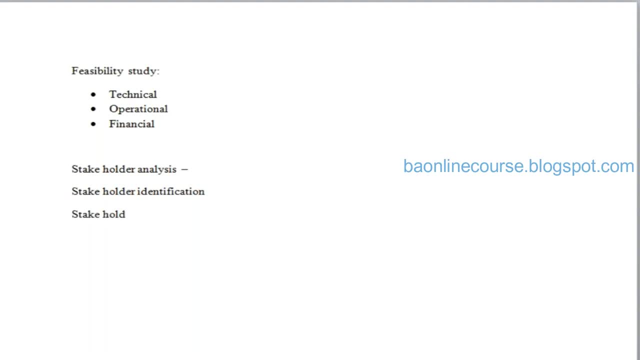 � displayedceu nausea you wouldn't even say okay very clearly one date salmon okay so I did well with that Okay. Second, we call it as stakeholder analysis. Third, we call it as stakeholder management. We divide this into three parts. We divide the stakeholders into three parts. 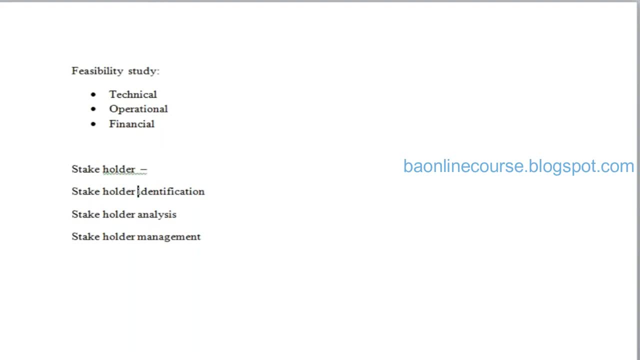 One is stakeholder identification. Second, we call it as analysis. Third, we call it as stakeholder management. So these are the three different types. One is about stakeholder identification. Second, we call it as analysis. Third, we call it as stakeholder management. 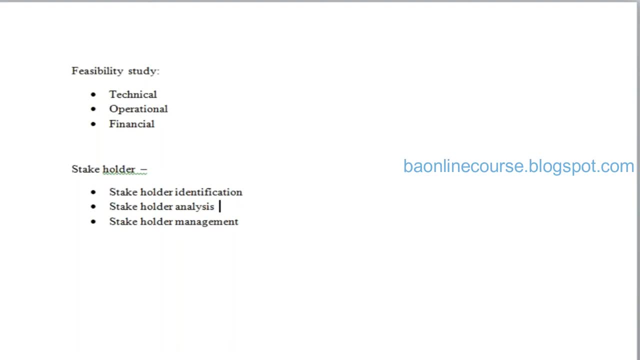 So three things. What is why are we divided this stakeholder into these three parts? First, for example, we keep the stakeholders aside for a while and talk about the stakeholders for a while and talk about other things. For example, let's say, you want to work. 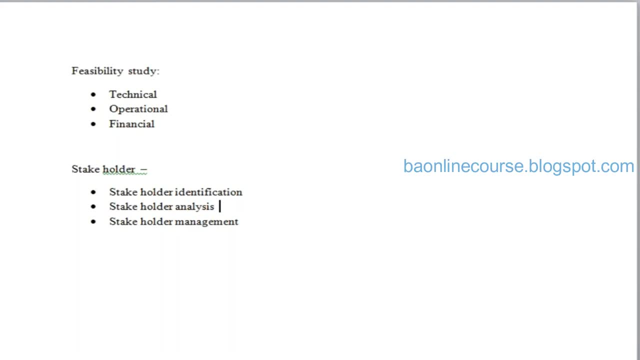 A work has been assigned to you. Okay, This work will be for around six months of time. You are the point of contact. Let's say you are the POC. So you are the point of contact. If you are the POC, will your decisions work? 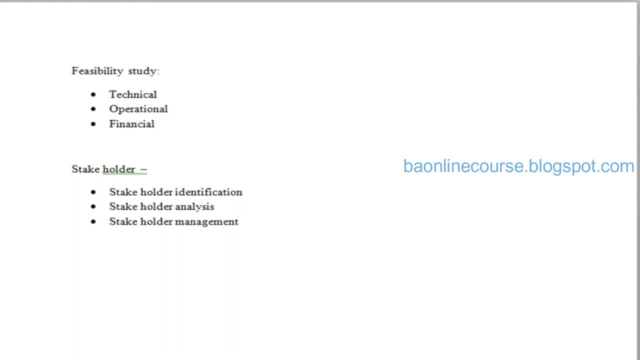 Why? Because there are n different people who directly or indirectly influence your decisions, Right, Right. So what you have to do is, every time, the employee, especially the employee's responsibility is to manage all these. As a person who is working as a point of contact for some assignment, you need to coordinate everyone. 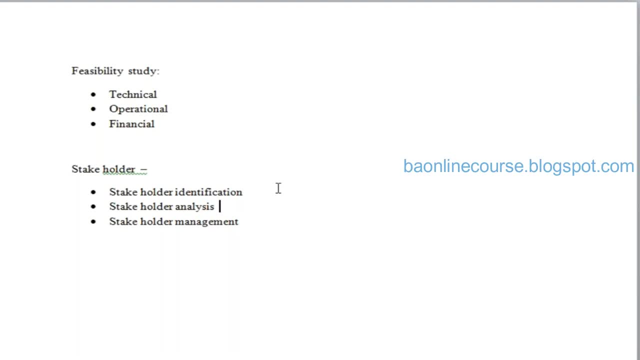 You have to coordinate with the POC and work with them. To work with them, first of all. what do you have to do? First of all, who should I talk to? Who should I influence? Second of all, who should I identify? Who is your boss? Who is your boss's boss? 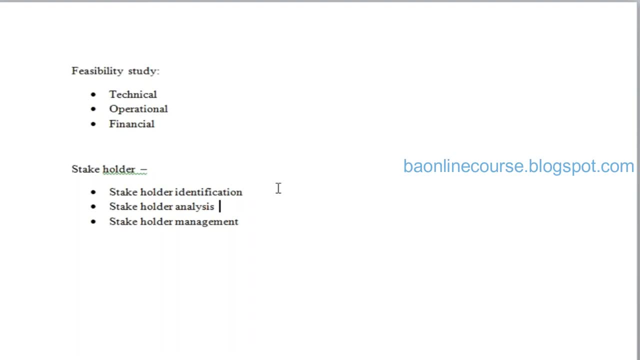 Who are your subordinates? Who should we consult? What should we talk about? You should have this clarity. If you don't have this clarity, you won't be able to work Right. Yes, After you start your work, you won't be able to find out who to consult, Right. 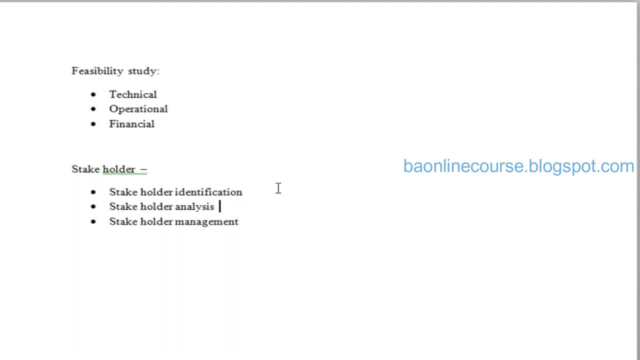 Yes, That's true. What will you do Before you are starting the work you will finalize to whom I have to discuss with? Yes, Is that right? Yes, That's why, wherever, whether it is a regular work or a project- 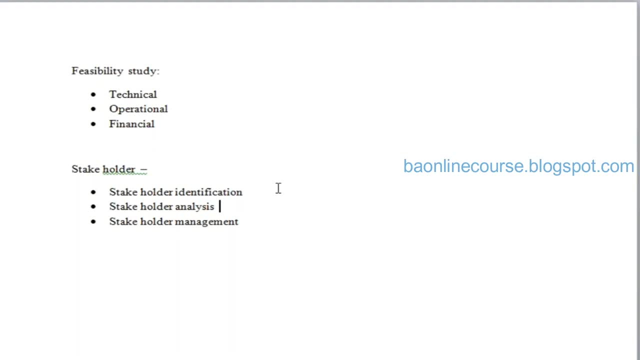 stakeholder identification is so important. for any of the projects, Stakeholder identification is important. What is meant by stakeholder identification? Stakeholder identification doesn't mean identifying a list of stakeholders who are required and who are responsible for us to manage forever, Throughout the project. 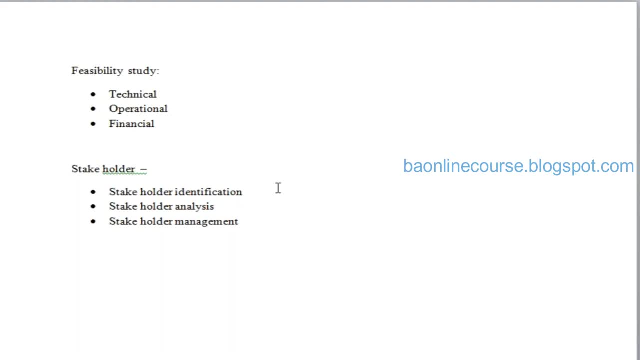 How to identify them. There are 100 people, Right, There are 100 people. How can we manage 100 people? practically, It's not possible. Okay, There should be some strategy, Right, Even if there is a policy or a strategy, 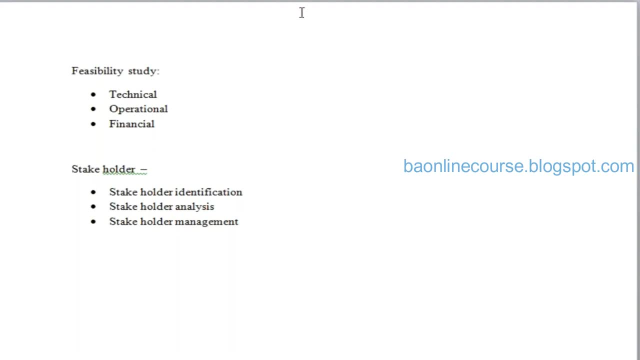 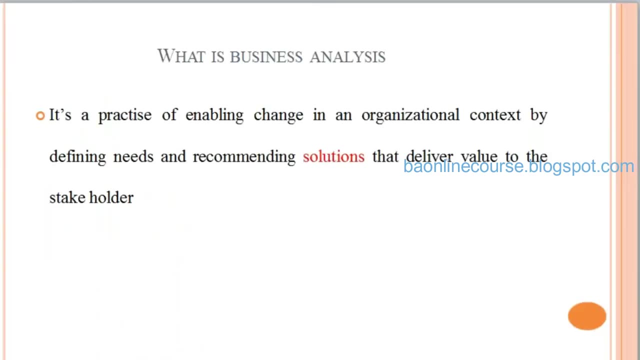 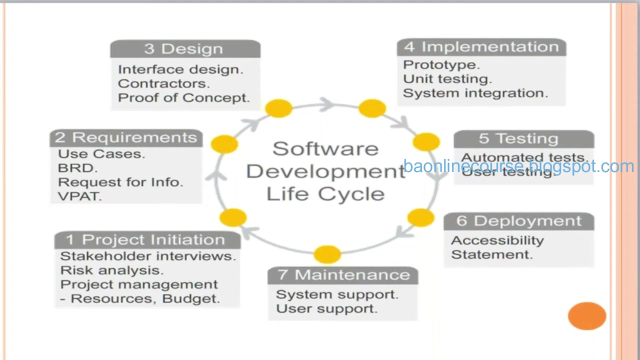 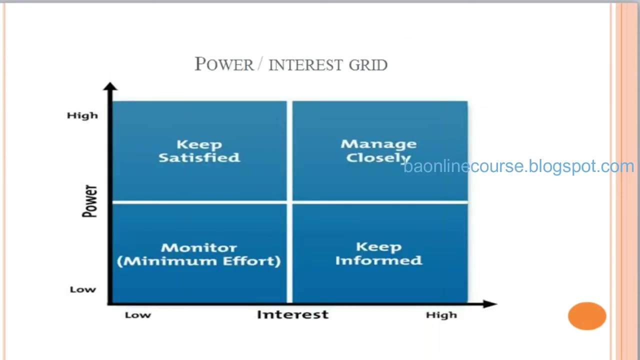 it is possible to manage all of them. For that we use a matrix called Power and Interest Grid. I will explain. This is what we call it as Power and Interest Grid. This is used for stakeholder identification. What does Power and Interest Grid mean? 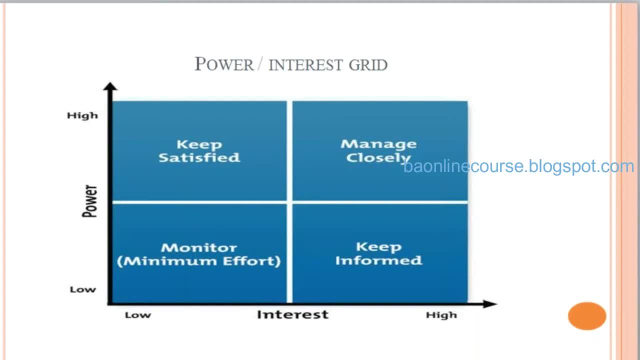 It means who is in high power. How do we do this? X and Y axis? Okay, We divide it into X and Y axis. Power and Interest, Two, Two different things. Okay, We divide this into high and low. 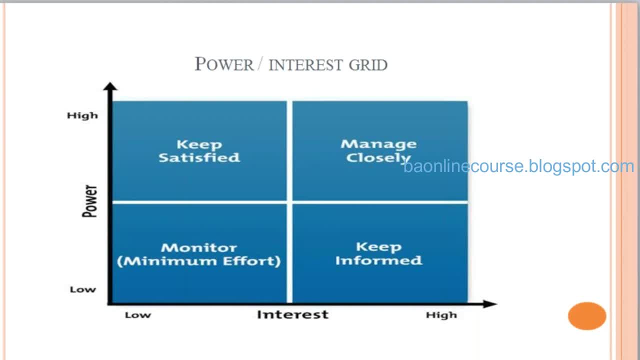 Interest is high and low. Power is high and low. We divide it like this: People Who has low power? They are low in power, They are low in interest as well. How much do we give them? The effort we put on them is minimal. 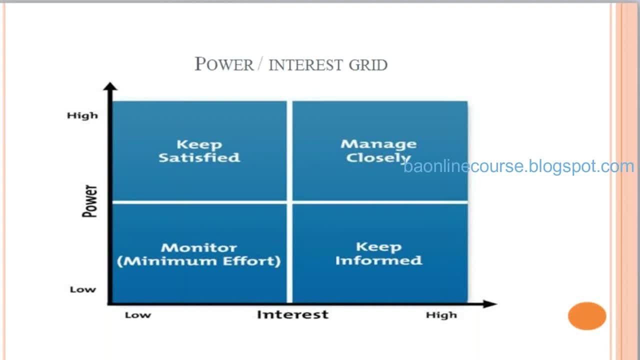 Just monitor them. That's it. We don't need anything. And if they are in trouble, we don't need anything. Okay, What? Yeah, Yeah, And next. I am hearing this: Yeah, Thank you, And next. 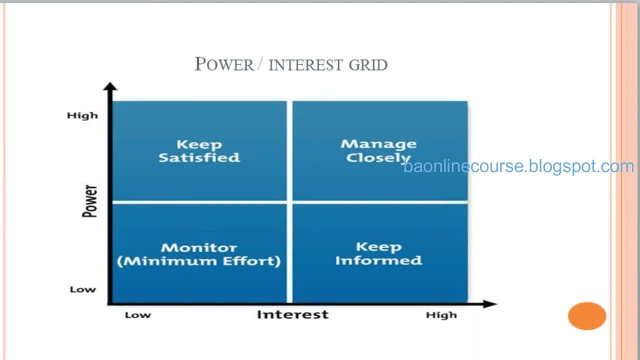 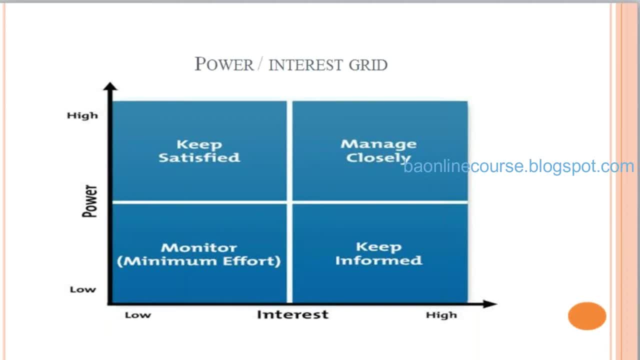 You need to inform them. You need to inform them In Regular intervals because they have more interest. Even though they have less in power, they have more interest and responsibility. That's the reason you need to inform them in regular intervals. How do you inform them, Alindi? 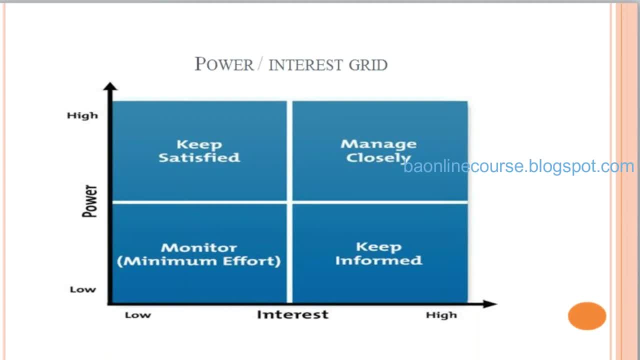 Whatever the changes, whatever the decisions are we are going to take, Whatever the changes are we are making and all that You know, whatever the decisions are, information is given to them In the second category. Third category: people are nothing but person who has high in power. 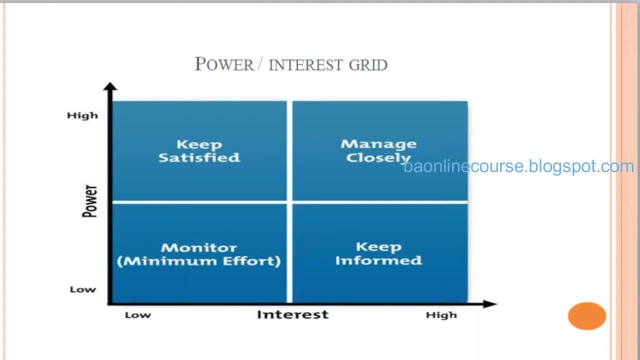 Low interest interest. you have to manage them closely. you have to manage them closely right at the same time. a person who has high in power and high in interest. you need to satisfy them forever, because these people might be business owners or IT heads or functional heads or something ever in a couch, okay, so first of all, 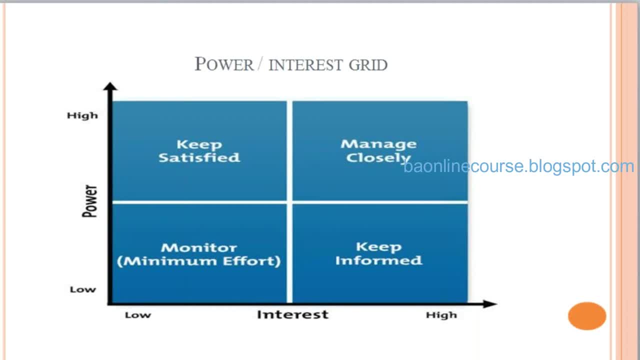 identification of stakeholders is important. so once you do just high current identification and all we have to use this power interested to cross check. and they high power and high interest. no power and no interest. no power in high interest, high power in low interest. understood, yeah, mm-hmm, this way. 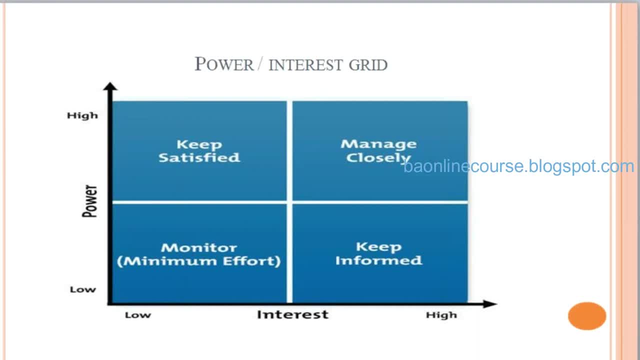 you have to streamline and this way you have to identify who are important and who are not, and take an important and take how suddenly the near government, this you are in, the entire human, and deal chiality. the point here: and yeah, mm-hmm right, regular changes will make regular requirements to make ever so many. 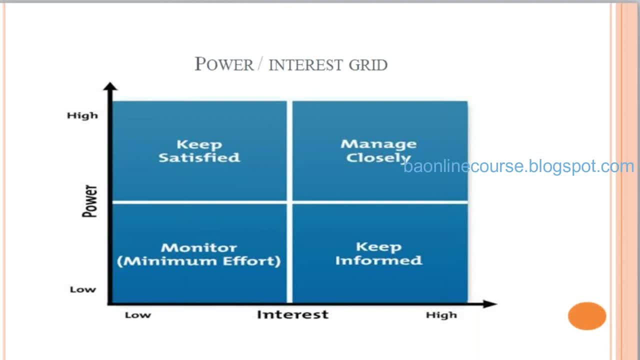 market and project manager to market, you're gonna. project manager is responsible for the project. okay, honey, business owner, you put up with a power line, can you regular them? it actually, today he also live because, whenever it is required at all, that time only remaining procurement, even this. 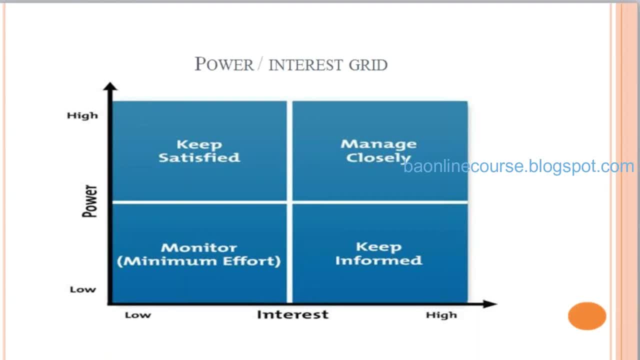 different rate with the number of budget issues on those, the procurement income in a matter. so when I mean, yes, the moon, first of all, stakeholder identification. we have to do for that. we have to, we have to and I analyze it, you right, we have to analyze who are all important in what they are. they're. 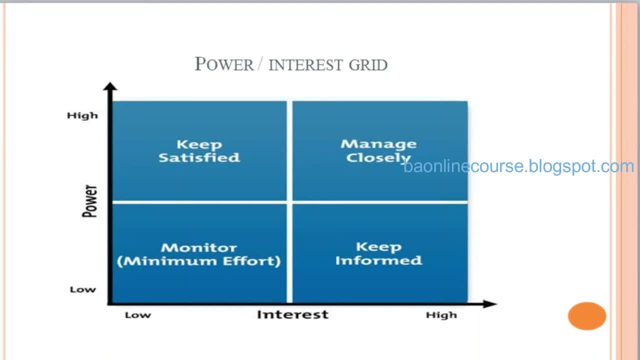 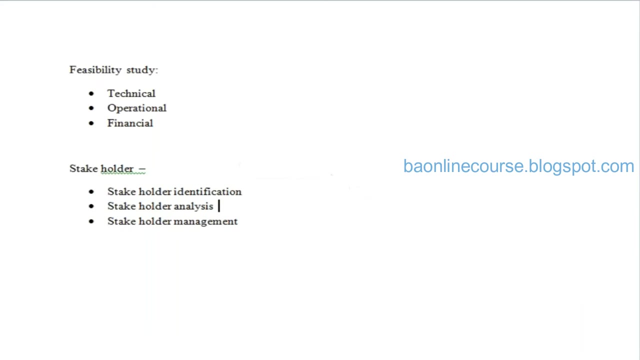 important, amazing. we have to. what are we doing? we were doing stakeholder identification. this is the first. okay, yes, once. once the stakeholder identification is done with, we are going for stakeholder analysis. what is meant by stakeholder analysis? stay behind analysis doesn't mean not. 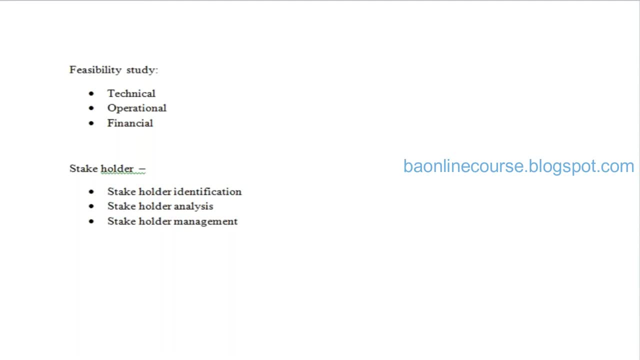 check it. okay. stakeholder analysis is like no identifying who are all critical to the project, like know whom you should be able to identify Jesus already my ID- we Jesus and the identification IP one, unless he and I let's hear to do this. take all the analysis and all. we have a matrix which we call it as RAC metals. hmm, 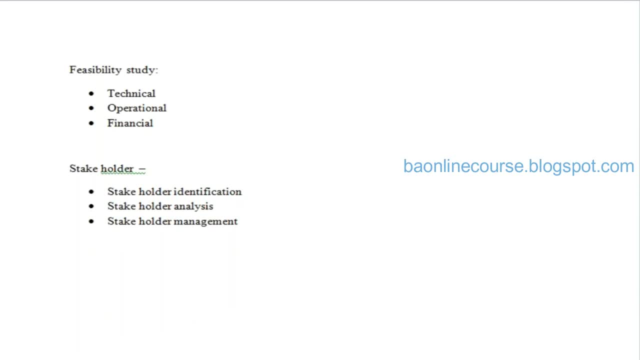 We have a matrix called as RACA matrix. This RACA matrix is useful to analyze and manage the people forever in one day job. This is not a one day job, right? This is the kind of job you have to endorse, or you have to understand, or you have to follow. 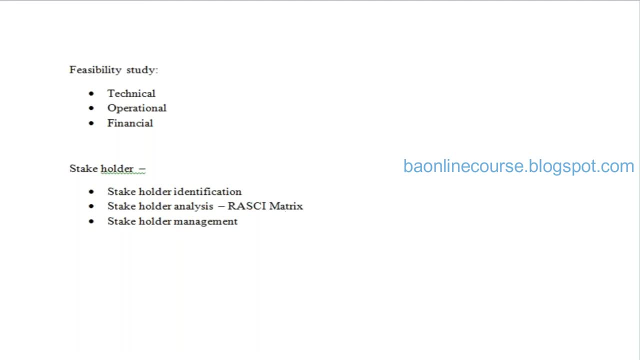 throughout the project, and throughout the project I could give you a little concentration pattern. So, Banaki, the kind of analysis and access to manage the kind of matrix, what we call it as RACA matrix center. RACA matrix center: It stands for responsible, accountable, support, consulted, informed, responsible, responsible. 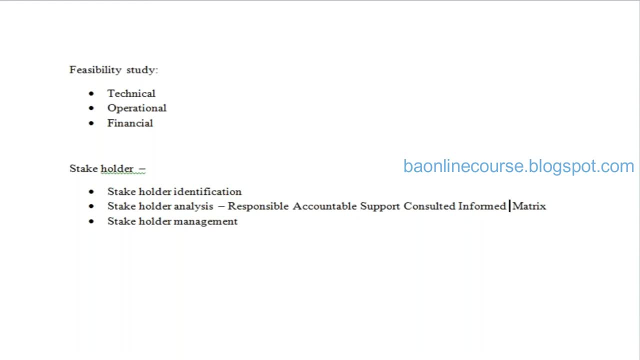 informed. You can identify the stakeholders and use them for RACA matrix in this stakeholder analysis management- How to use it. I'll show you Stakeholder analysis so that you'll understand One minute. Okay, Okay, Okay, Okay. 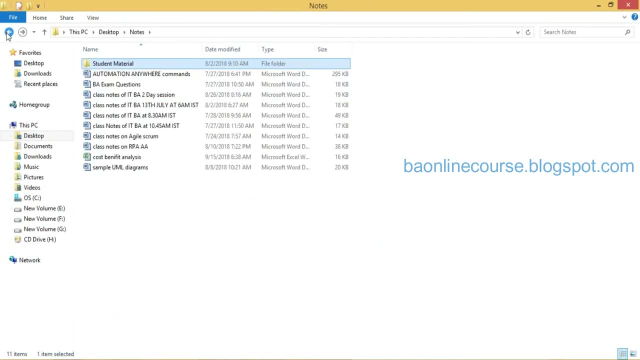 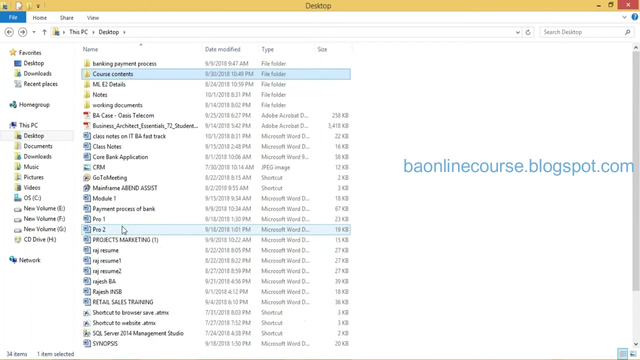 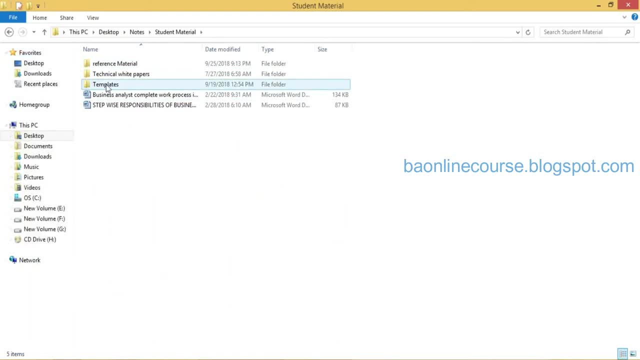 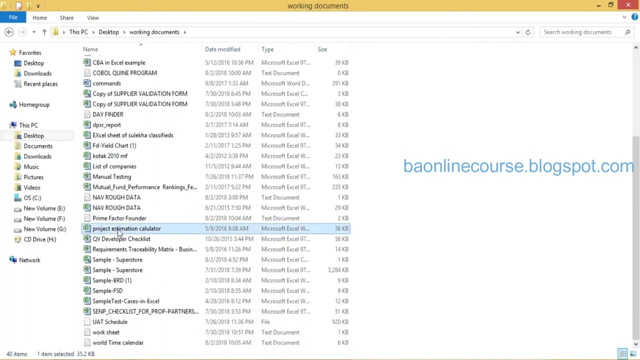 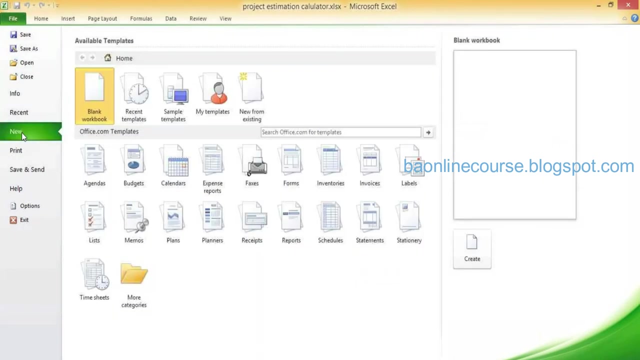 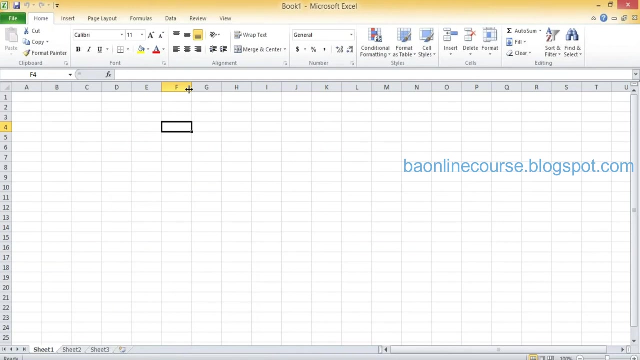 Thank you Exp」. Bye-bye, Bye, Goodbye. So the next one we just need, just okay, so it allows us to take stakeholder analysis first- is ID number: Okay, Task Okay, What type of task is this? Okay, Stakeholders. 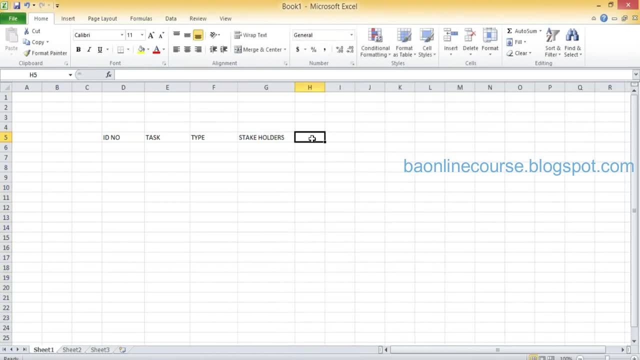 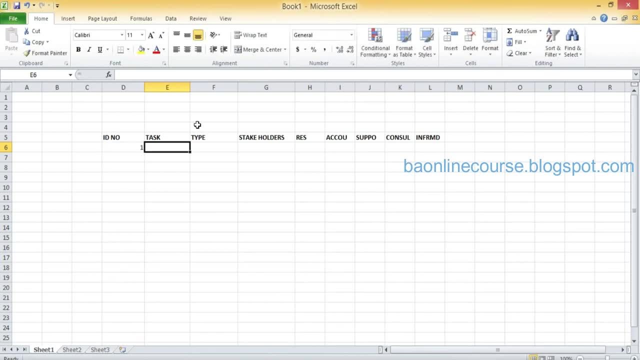 one example: children jacket ID. number one task in P: user interface designs: user interface design chair in the type of: what type of tasks is this? it is about friend. is a friend pages designing center? okay, we are designed. so your interface design is in the type of stakeholders name. another we have to. 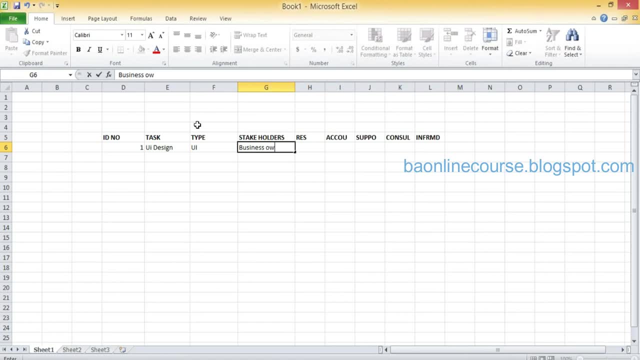 list the stakeholders ever in ideal pages and, for example, business owner, IT owner of a functional head. function of a subject matter expert: okay, look, procurement team team one of the project manager, none of the be a. okay, developers, so the a designer, so your designers from target mm-hmm. testers, we learn more. I didn't pay a song. okay, I in case we'll get a. 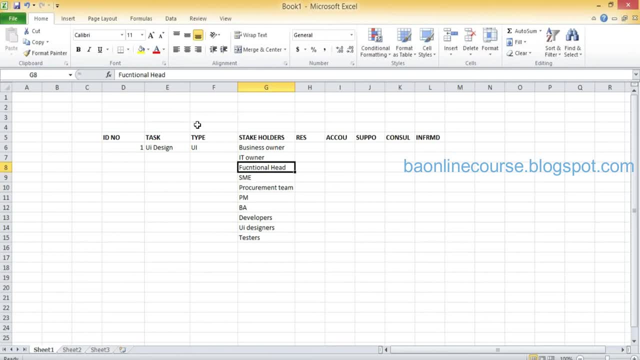 cone. you can arrange us, not a you. a design business owner is responsible for that. he's an easy accountable for that. no, you can arrange us, not a you. a design business owner is responsible for that. he's an easy accountable for that. no, he support is required for this, not. 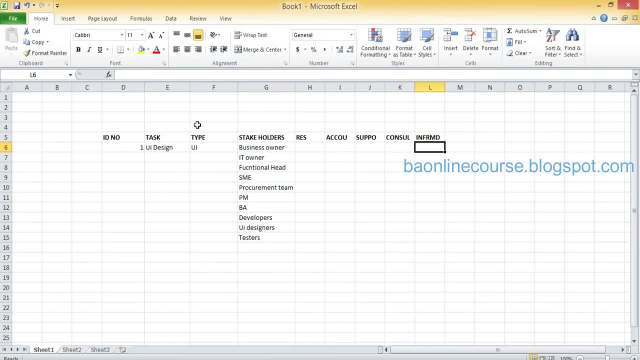 he. support is required for this. not required. consultation is not required. it required. consultation is not required. it is not. but information for a design is not. but information for a design. stand on it is not because you know this. stand on it is not because you know this one that has to do with all these. 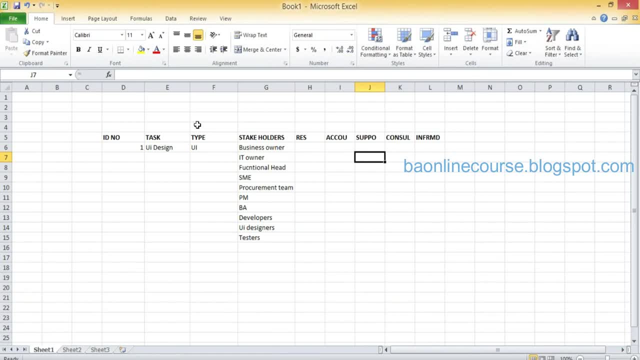 one that has to do with all these designs, and yours is good Arizona designs and yours is good Arizona. IT owner will take care of functional head. IT owner will take care of functional head. may not be one good subject expert. may not be one good subject expert. subject matter expert support might be required. 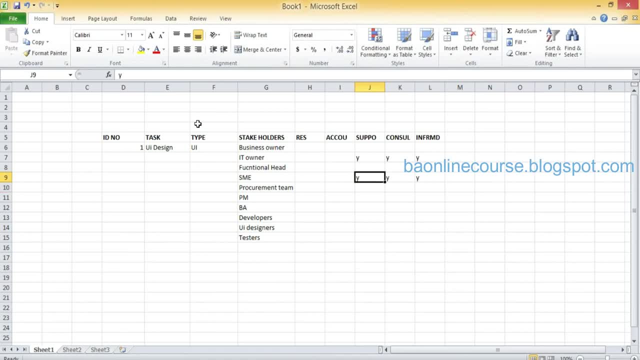 subject matter, expert support might be required, consultation and information to be be submitted as well. in the same way, when we are talking about project manager, BAs, and all it is required, even for it is for the BAs and all it is required, yeah, I think now a personal family. they work openly for you. what? 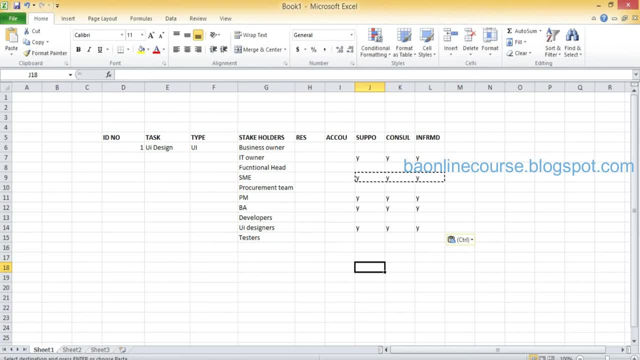 about testers. it's just we are designing trade and designing testing. we are not designing a lot initially. you're doing okay whenever the changes are happening in your designs, and all that time we might require some kind of quality testing and all everything might be testing. testers might be required. 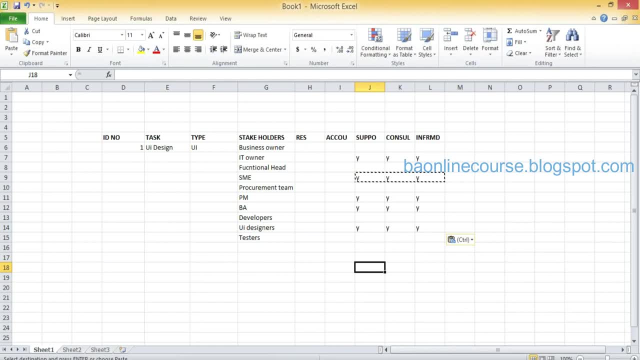 initially for your designs. initially, we are doing- we are not doing- any testing and initial information. are we sharing the home? you have to share all this information. you need to share this information with the us industry. clear hammer. yeah, it's a monotonous topic. different, different tasks, task to task 3, task 4: 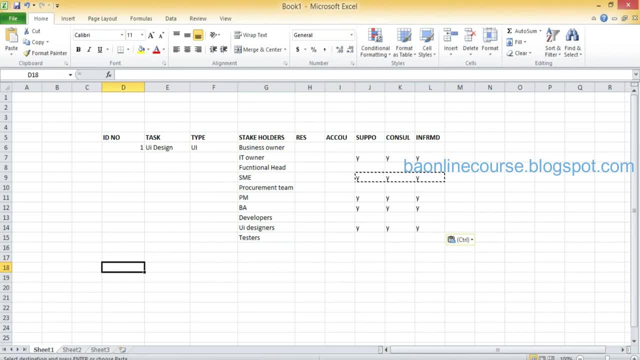 task 5: this usually manu intend a HP ALM tool and it's beyond the ALM tool. look right, I ALM do, love it may just aren't a predefined this bit test control projects generally predefined a spit contented in the auto-generate out. 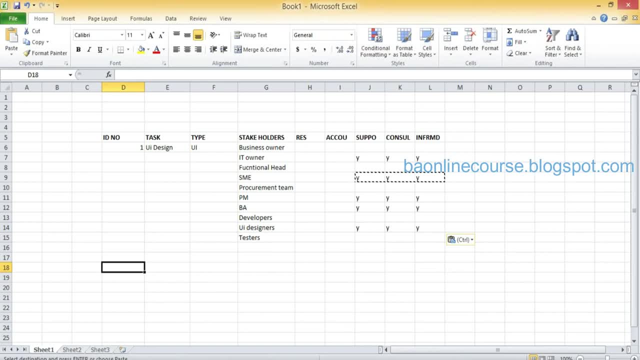 of the intent, a regular that you already predefined a spit content and came up to my day every time is: take order management throughout the project. run a boom, understood, yeah, mm-hmm. so this is what the importance of stakeholder analysis, followed by mr yes, stakeholders we are dividing into three. 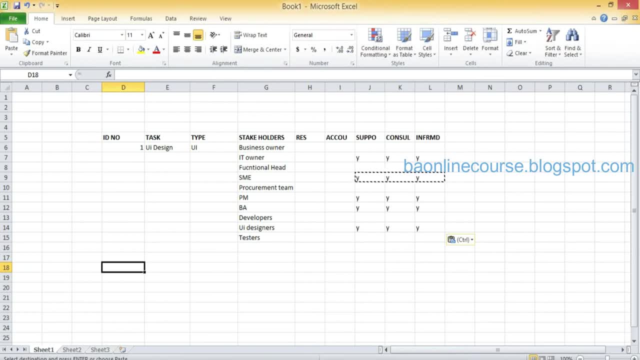 levels. one is an identification, so I can be called it as analysis or be called it as a project management, a risk management. learning is analysis, and then a continuous analysis and then a feasibility study. yes, the project management. you have to think about the reason that there is an analysis and 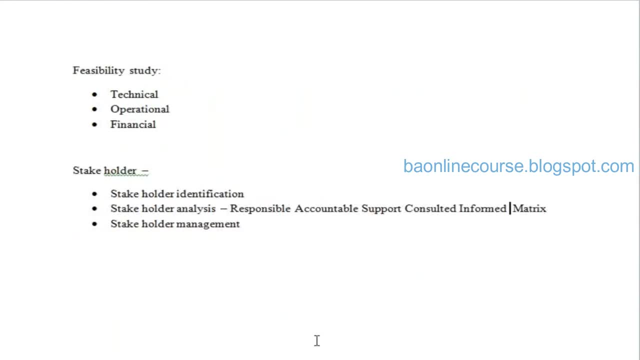 the number of people that has to be done. so the cost of the analysis given- so it's basically the cost of the analysis- can be done by the Executor, and this is what you want to know. the cost of the analysis and the cost of the analysis, because you have to manage your project- is community management right? the 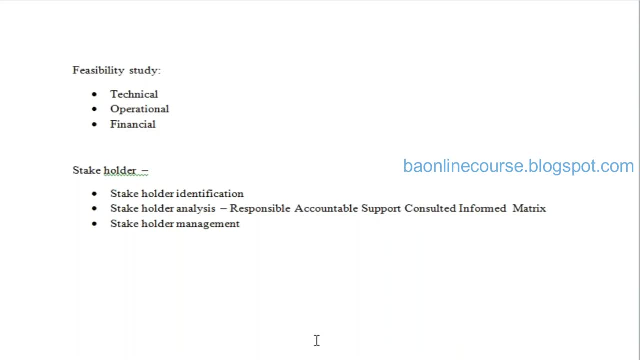 responsibility. so you have to understand what is the cost of the analysis going to make sure that we are not sharing any information about the project. and so you talking about requirement gathering and number how many next level of requirements, requirement gathering and everything what comes into the next level. understand, yeah, 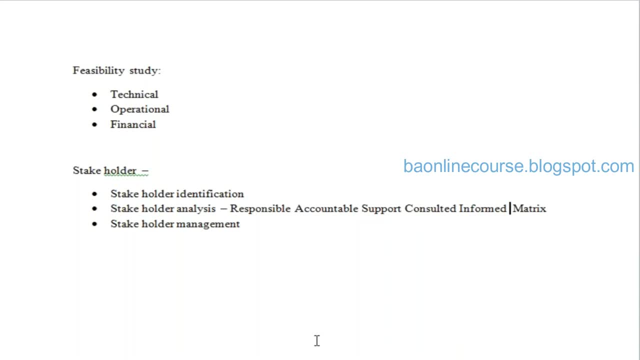 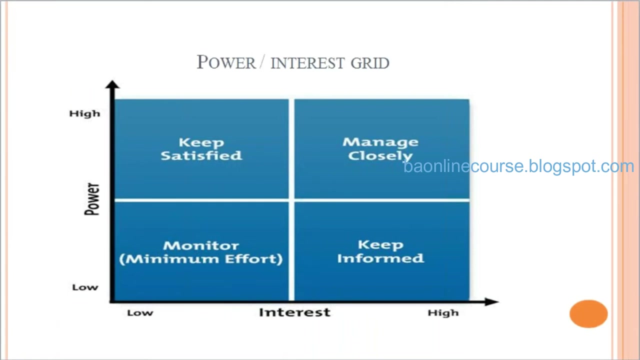 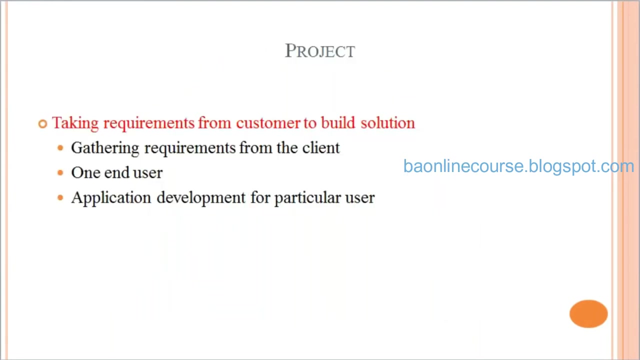 clear. so this is what is the first layer for any of the project. so, before you are gathering the requirements in order, this is what the major job of a business analyst, irrespective of the type of the project they are working on. okay, project, this is mandatory. but as far as the role of the b is concerned, 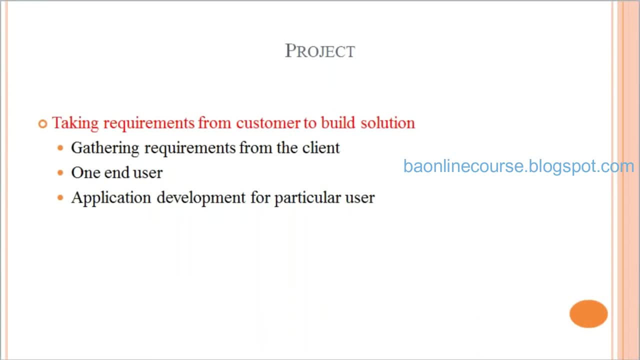 as far as responsibilities is concerned, you will find changes between the project based and product based. companies render, call companies. look at the project based and don't render. what's the difference between project based and product based? what's the difference? project is project, sometimes it's an application, maybe product itself is a product, like you know. 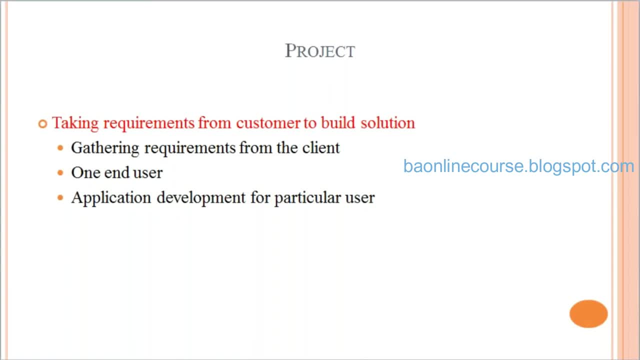 any, is that right, sorry, product key project key money difference: major difference: project key product key major difference in today: project based company client requirement, client requirement for carbon dollar. just project based companies enter and if the client will not do client of the requirement, which i do, we are working on the plan. 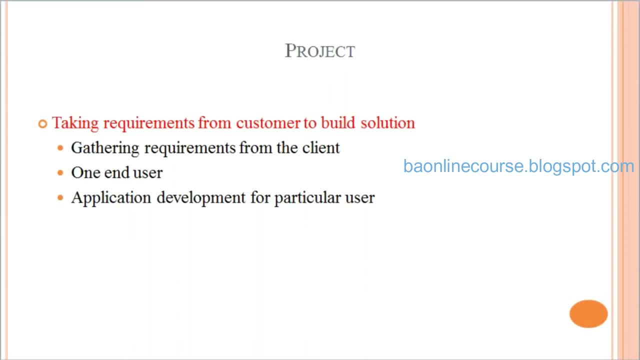 project. you are doing yourselfub some market research and you are developing some projects. you are developing some project you using for developing some project. first, this is what generally we doing: product based companies, product based companies, products, what kind of product you find? you see it this way: 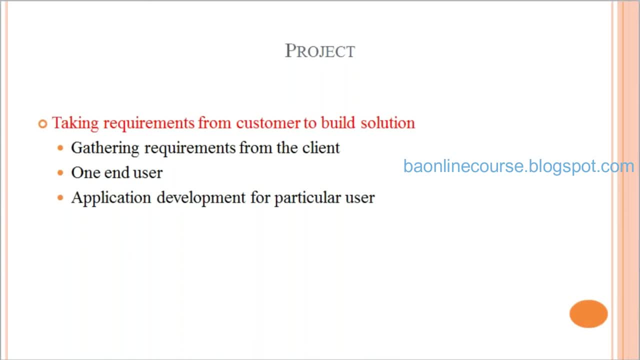 develop. just when we are developing the product, you don't find any client side product. a lot just not done for a while. the client was a yes, he is after difference. you don't take in forces with protease. is all this? consider as project-based companies Google and you will be Microsoft, done in the article. 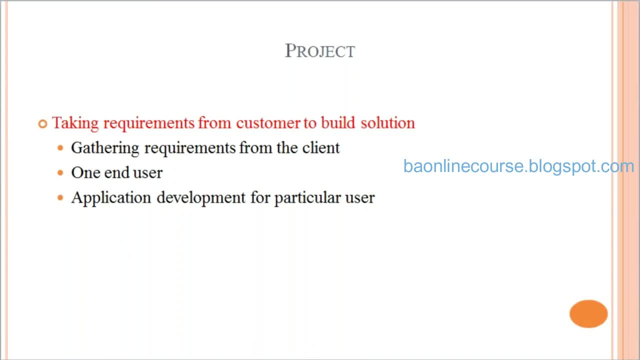 getting when they put up people's up to that Monday, I said you got even they would a we could product based on us and that a lot of products and I- he products were different, different customers, key for this sales. yes, I don't want to be services for this then, yeah, understood. 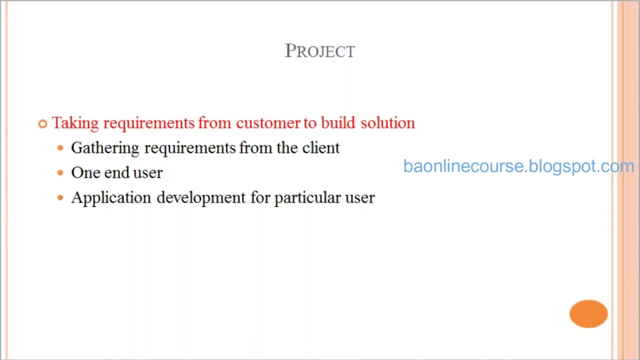 and it doesn't mean we provide a key in forces, for, like, separate products live under another. it's been a project development. don't know the product development around this, but he made a difference between the project based and promised you know what circuit. you can ask me one thing then: what is my role? 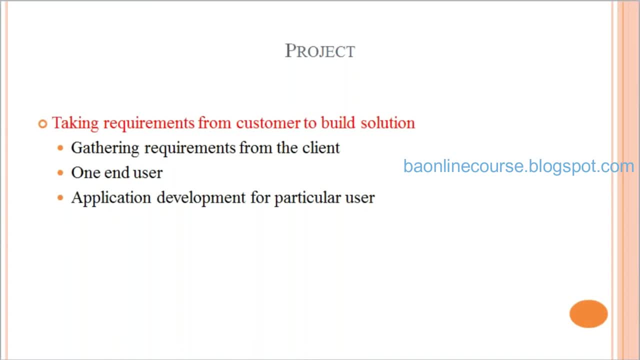 there right. so, as a be a, my job is to gather requirements, cover and the lies in between business and technical communities, project-based identity, product-based internet, and I can't even the entire, whereas in the first case of the project-based companies, you have a client if any difficulties and 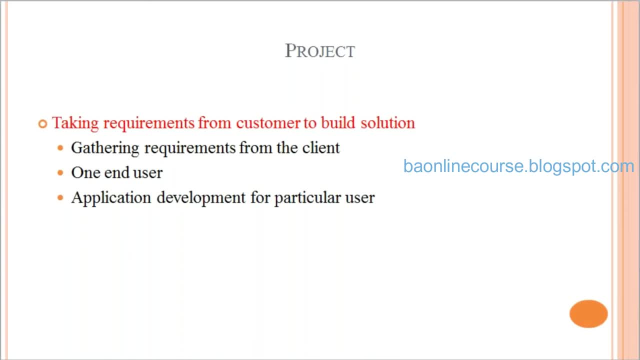 challenges you face and all you can interact with them, whereas in product-based companies you don't find anything else. we call and our customer, product-based companies look in the door because you have to create and sprint through your process. you cannot go for yourself as you don't. 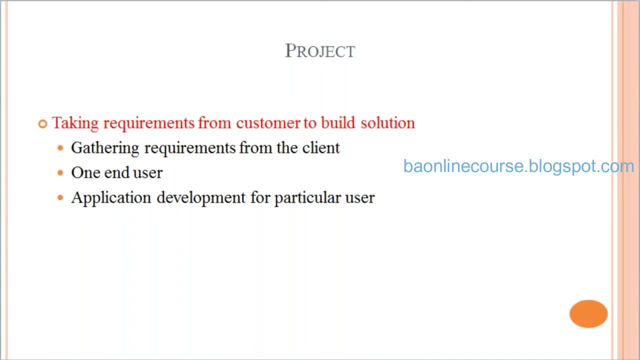 have any client something successful. It is very difficult to work in the service segment because we don't know when the client will call and what are the requirements. We don't know when the client will call and what are the requirements. We think about the limitations and challenges. 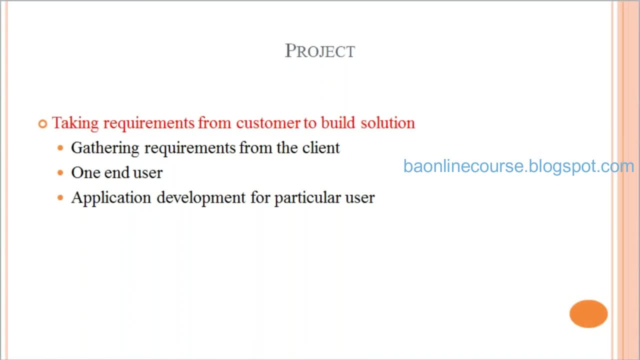 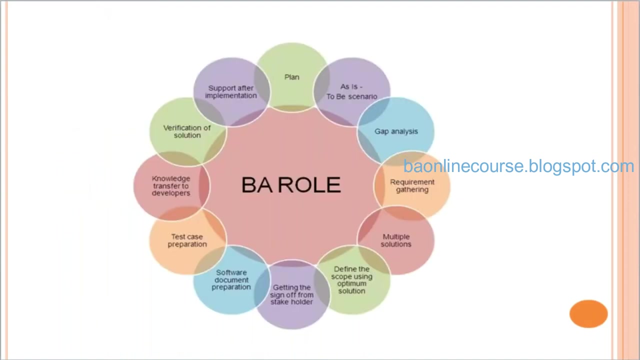 But the role of a BA from project to product. this is the difference. You can see that. That is what we call the difference between project based and product based. Clear, Yeah, Right, Yeah. So these are the roles of a BA. 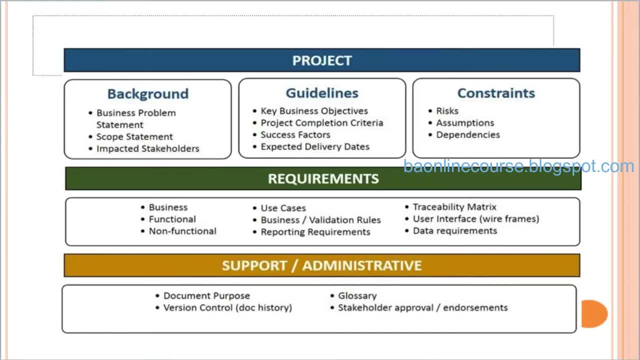 This is how generally the project looks like. Any of the project looks in this way. First of all, we have to do some background check and all that Background check first of all. What is the business problem, Right? So what is the scope statement and all that. 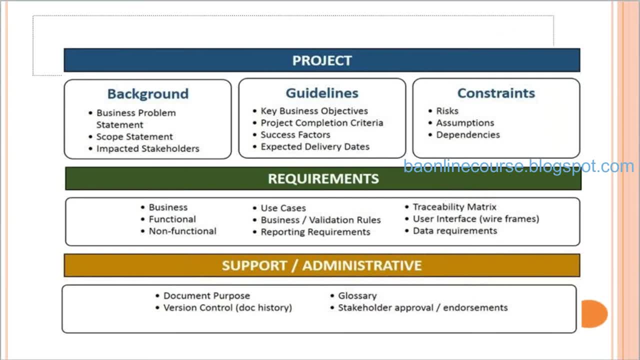 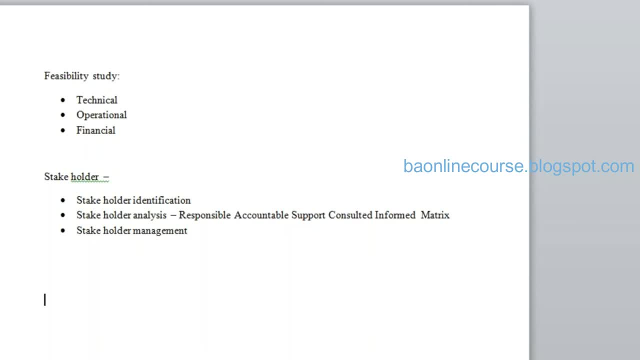 So whenever you want to work on the project, you have to follow three major points. Those three major points are as follows: One is about objective. Second, we call it as need. Third, we call it as scope. Right, Because we call that objective? 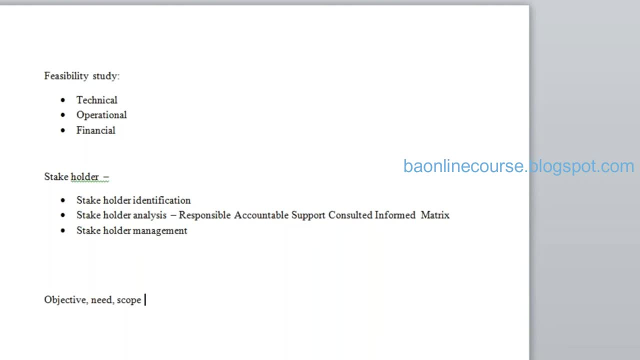 Second, we call it as need. Third, we call it as scope. Hear me, Yes, Listening, Yeah. So first of all, we have to understand the objective right. So what was the objective behind? to develop the project? So, if you want to understand the objective, 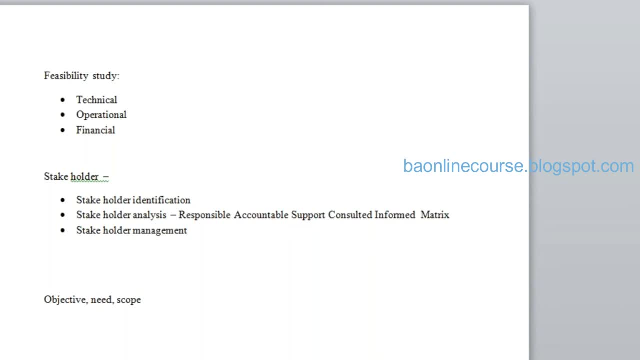 understand the objective behind this. you need to understand the business problem. so that's the reason. first and the foremost thing we do will be called as a business case document, and business case document is the most important point in project development. what is made by a business case document? business case document is the one which explains you about the preliminary levels. 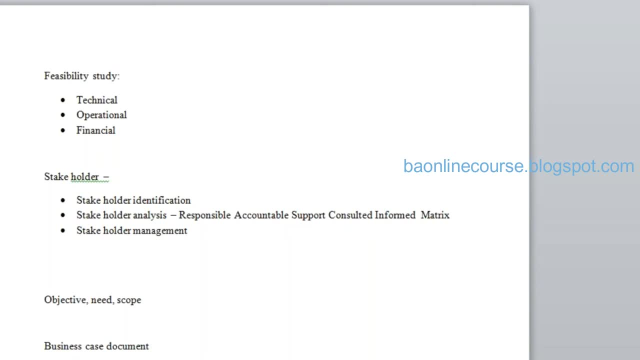 of the project, what exactly the problem is all about. okay, how big is this problem at all? so these things to investigate that we have to prepare a business case document. so business case document for you and the initial guarantee before you are going for brds, and all that. 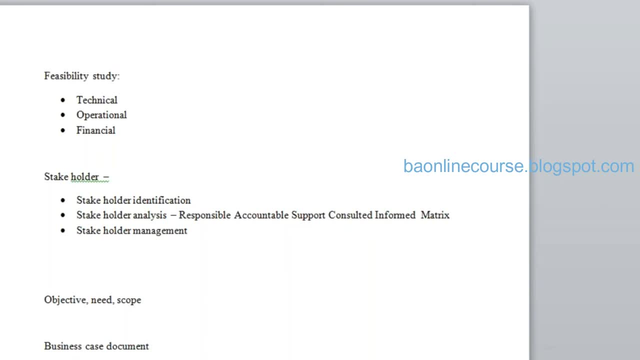 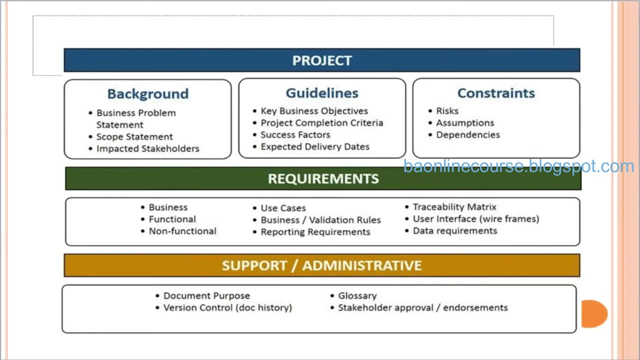 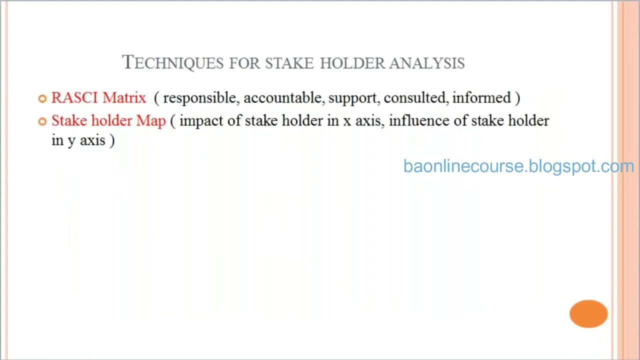 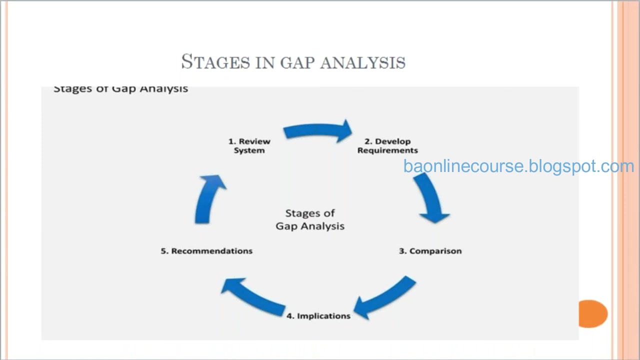 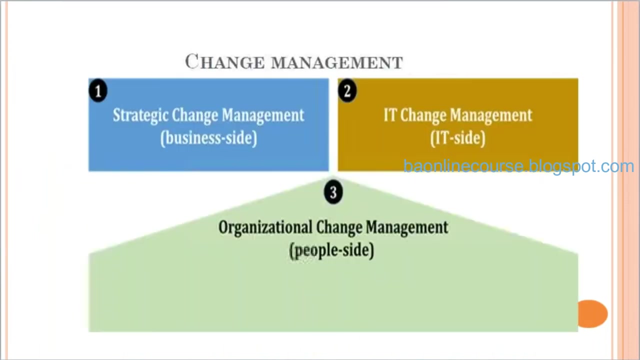 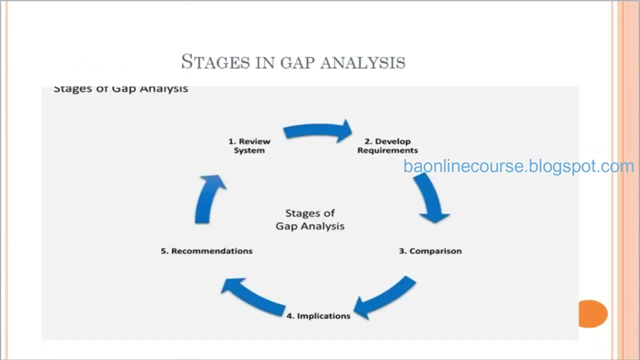 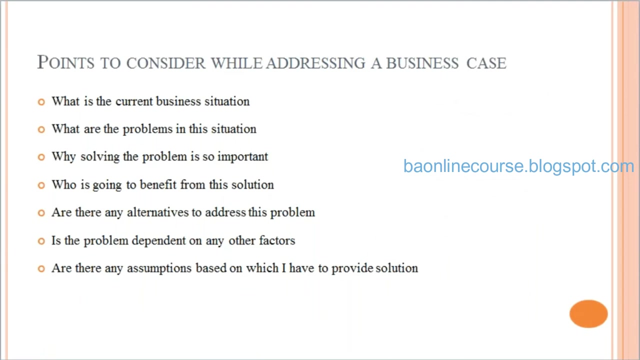 what are all is required for a business case document? there are two points we have to consider to address the business case document. those are all as follows: just and just one minute hammer, yeah sure, so right. so these are the points we have to address when you want to. 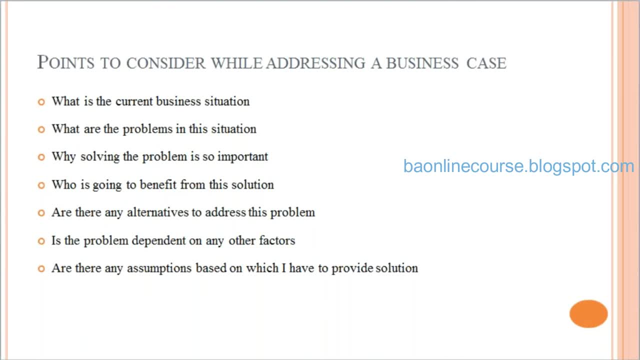 develop a business case document for any of the project. so the first point is: what is the current business situation situation? second, what are the problems in the in the situation? third, why solving the problem is important for us. who is going to benefit from this situation? what are the? 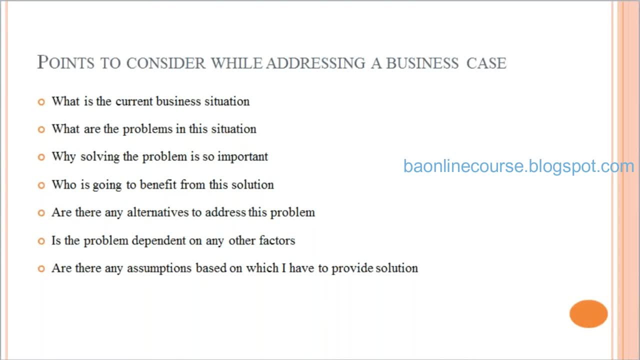 alternatives to address the problem problem. what are the dependent factors which are connecting to the problems? what we have identified, followed by this: what are the assumptions we have to make to provide a solution for this understanding? clear mm-hmm. so these are the points, and then we are preparing a business case. 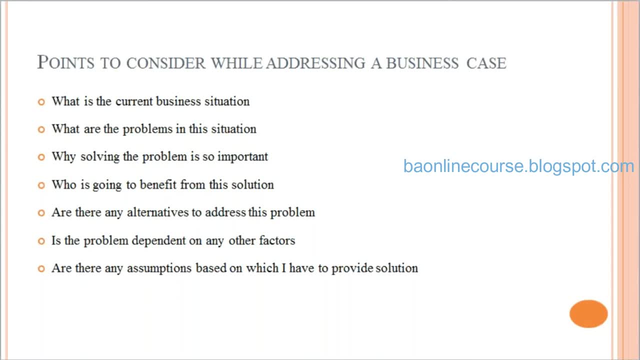 document. so, irrespective the client, irrespective the technology, irrespective the domain, unless and till. if you don't have a clarity on these points, it is really a difficult task for any of the BA to develop business requirements documents or something like in near future. yeah, yes, yes, and these are the 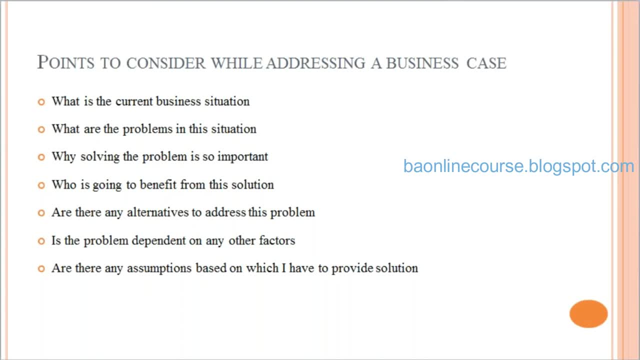 points we have to consider in irrespective of the domain, and they really care about many pre. they teach you know when they could. a generalized going in Japan. okay, it is not only relating to health care and it is unconscionable. the plane to commit this problem. the address a on a. 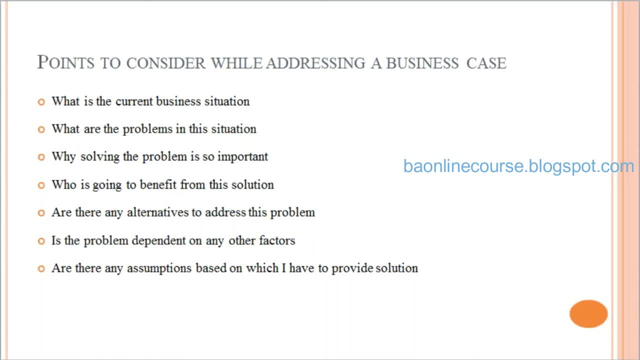 a first clarity of thought is important. unless and till, if you don't have a thought of clarity, it is really difficult for you to come up with some kind of solution. the solution should also be based on few assumptions. you can take the assumptions and dependencies and commentate when they 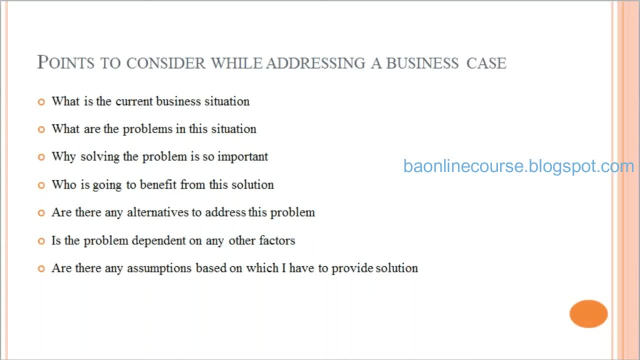 may problem. a solution to a lucid up when you shall go to it for pocket assumptions, secondary solutions and dependencies assumptions at the NT parameters. one at them we can tilt a matter: quality parameters. what other parameters we need when we are providing solutions? these are all were content as televisions. 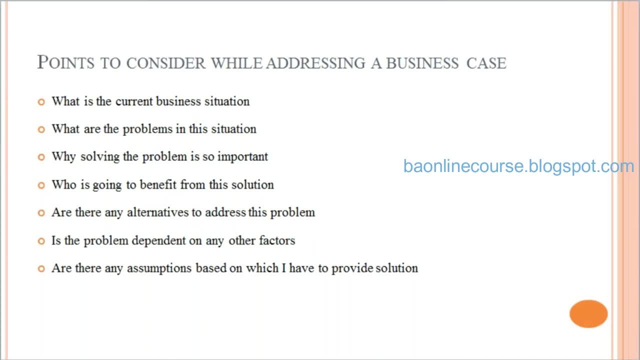 like we have to send something at least antique. this is how it could be writing here. he says what he mean happen and is much less ==. Yeah, look down, just watch a Twilight. this is what we are trying to retrieve in future for this. this is what this vision. that a graded option and simple like this. lately, mediator, I think so we getų müssen something. this is what we are trying to receive in future and for this this is what must be. yogurt side dish: advantage value is into something. specific solution. you no, look, I don't like a. this is not a word cut, nor is this real. you can, ehrman, because this isn't work. something smart, it cannot. 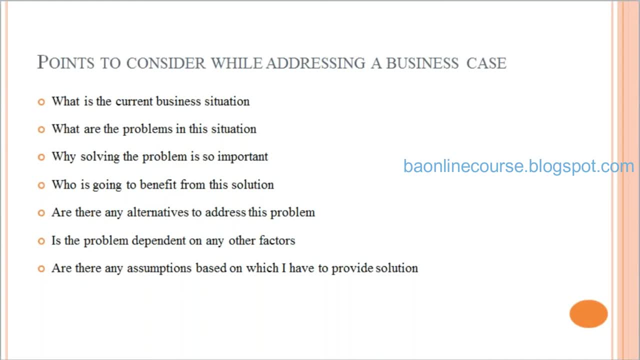 assumption. and second, we call it as dependencies. and what is meant by dependency? dependency doesn't mean he solution given me the dependency other, but only, for example, POS system. a matter of POS system near update, chat down, POS system, update chases are important that you update jelly along. 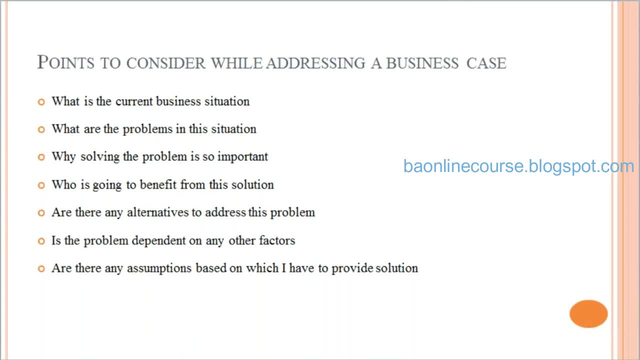 with POS system, you have to update inventory application as well. if you middle application on a topical therapy on day, you is application and judges now appear in a day, that's a wrong mistake this time. yeah, inventory application. a proper Galena POS are British marine year and 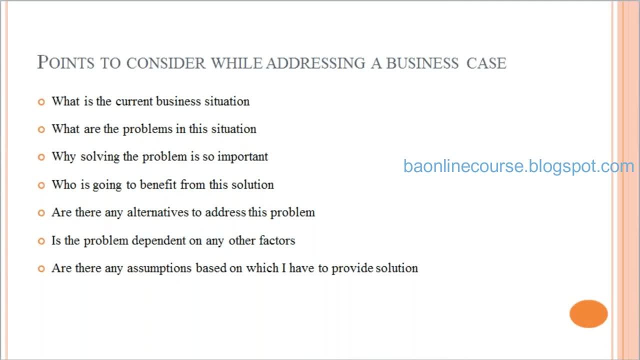 gay together miss barcode bit scale scanner with the barcode of the product scan. just a made it the mark for me. product screen display out from the latest mail to the because POS connecting for inventory, yeah, I, inventory application. a proper Galena and a day POS is a dependent on inventory and the inventory, hmm, and the proper Gondola maybe a. 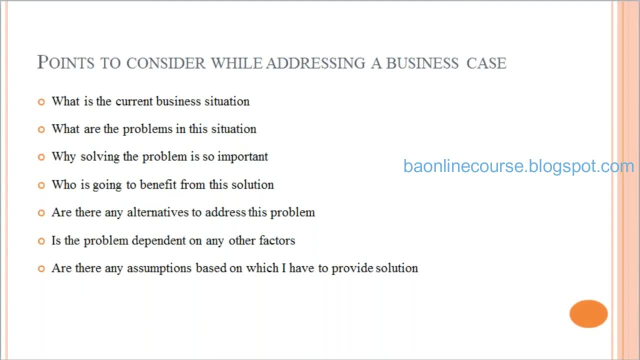 sister. so done in dependency and don't application develop chadwick. other the application case supported applications. a way to know you I'll be entire Cooper sector online is verification just for an, a man in dependency center. so assumptions and dependencies are both are two major aspects. 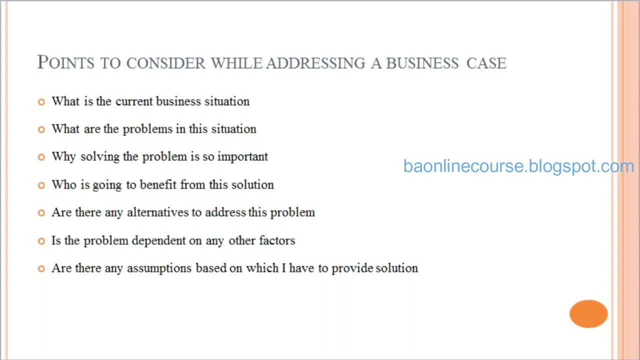 points. whichever is required for any application to develop or any solution to be provided me there is a solution, value and put a. you need to see the assumptions and dependencies as well. yeah, yeah, mm-hmm. right, yes, so once you have come up with some kind of 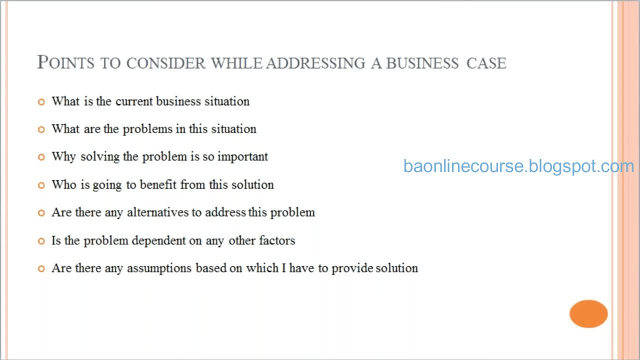 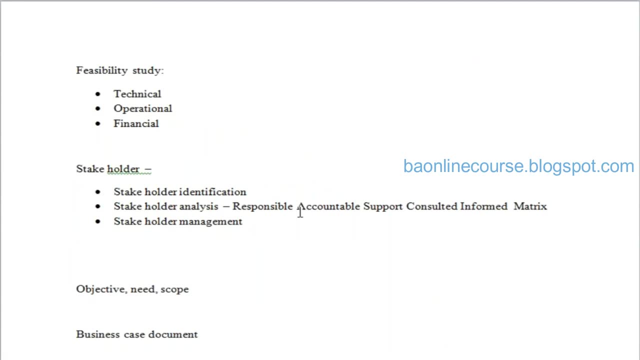 business case, understanding and all. then you can develop some objectives. objective one day. then you can do what is meant by objective. objective doesn't mind the one which you are trying to achieve. objectives in the grass quarter problem: there's pain in the government key, so usually change to that and they seem. 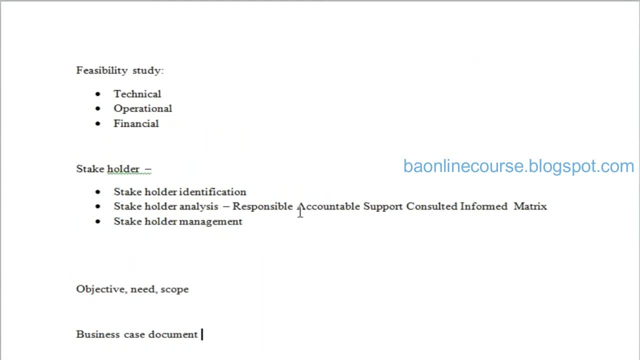 simple, simple without any victim, make solution rhyme and you know, cut logic. kitchen miss touches nobody and Jason of right now, I'm sorry to the mirror and I really started and correct going to start Jason and cut the ending. I could believe in ending me. just love starting in the cunning because you don't have a 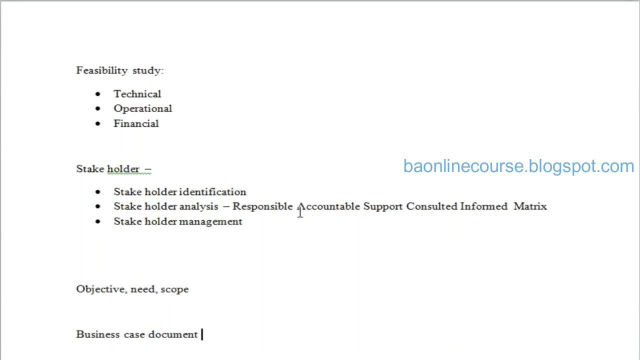 proper objective there, mainly what is my goal? and then make the little solution and to not the kind of goal makes the goal. the goal is the degree goal. airport, when they may start? you didn't correct. can I start, Jason? can even the influences and all slow the project me. 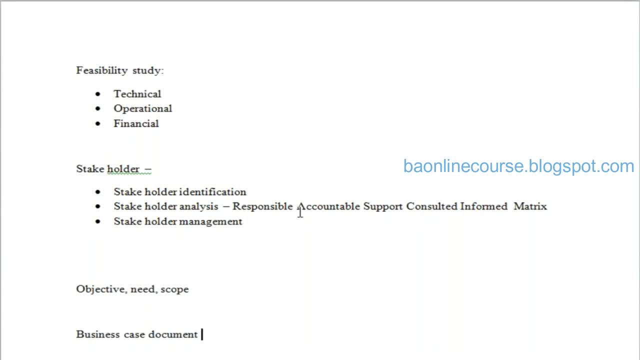 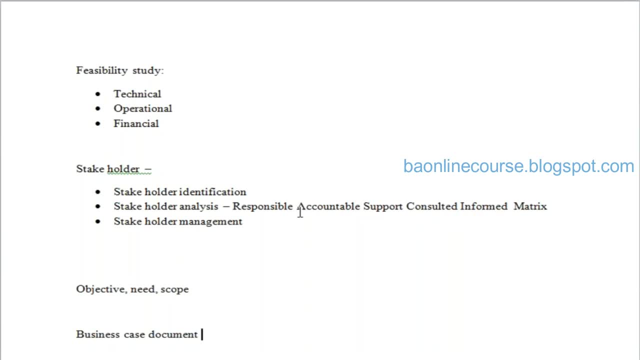 yeah, meal on the market shape. happy me examine when I was bombarding approval in. can't try and let me they MEAN cancer. yes, yeah, between time, Perth is to consider. you have to provide solution, me solution, private you set up. do you have some your own limitations and limitations in a matrix limit? call on a. 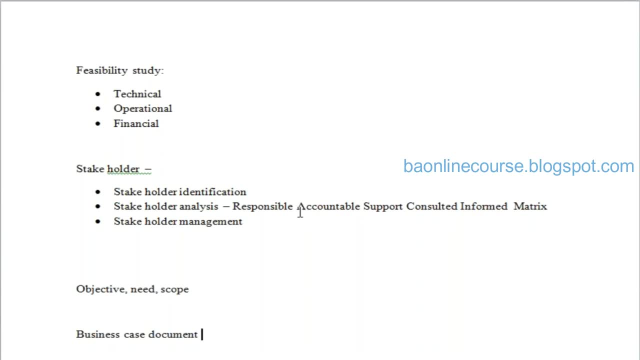 limitations will disturb it. call and day. you need to put some objectives and what is your final goal, what you're trying to achieve based on those up? is your problem solution? a miss, miss Daru, but not what client is expecting me understood, yeah, yeah, yeah. so objectives are important, so object is goal and all. 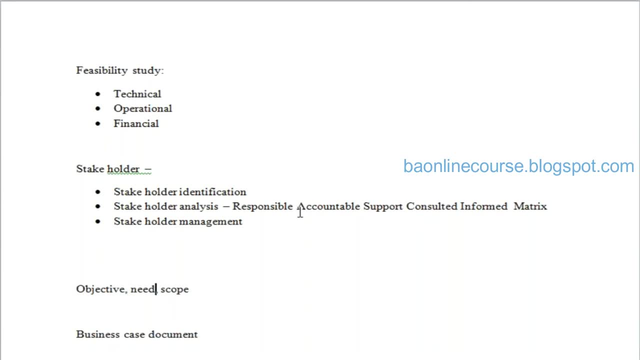 were important initially. so once you have done with objectives, you have to have to go for need. this is what we call it as need analysis. my client is asking us to develop the project. what was the required, what was the need? this is what we call it as need analysis. need an up to my later into category. 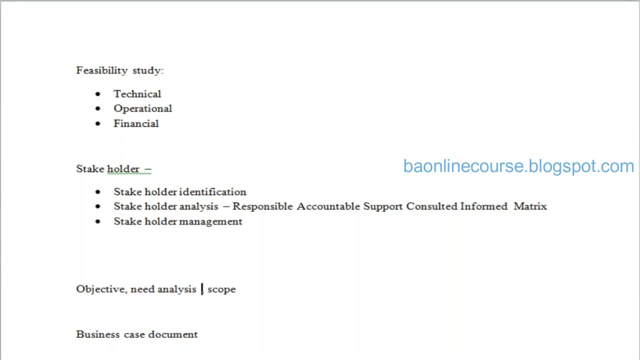 system need is in present or in future and you put it back right before. hmm, you put it apart and then the kind of strategy, what we follow will be different, important, the kind of strategy, what we call and see- I'll end a you need to have need. okay, next, once you have done with 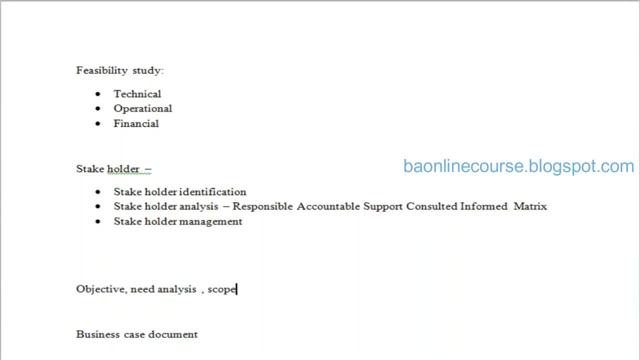 next, once you have done with next, once you have done with next, once you have need, you have to follow scope. what is meant by scope? scope doesn't mean the possibility, make on a time and make on a budget and make on a manpower. resources and Dean to volatility and requirements are not any chances in a we can meet me. 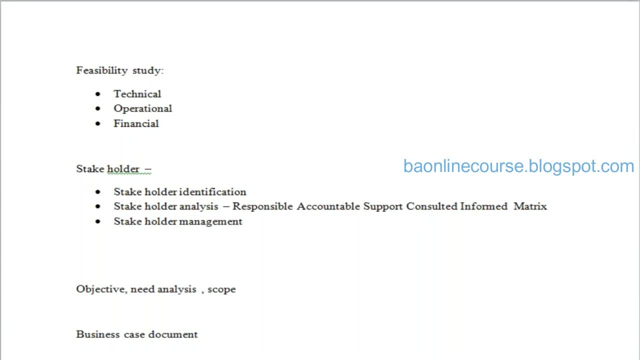 in a scope. can the rascal scope doesn't mean the possibility of working application monocular a challenges when they put on a scope. can the rastam go about the book and take Monica implement shared an account over a group? is possible team and a community or Japanese he or she up in the possibility in the 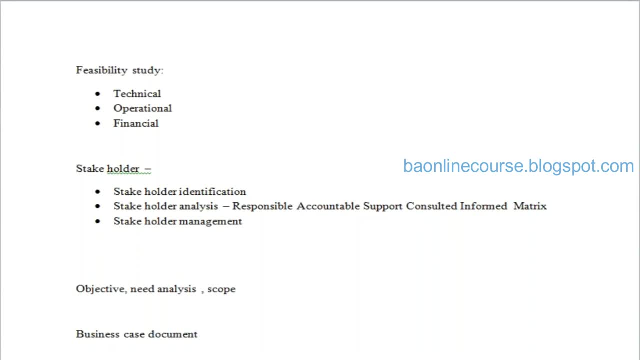 leader when they within time now, on a chain Galois, chase their technology monocular one more. they are within cost. low tunda a bit in cost level and underneath her, but a man for none. the guru da lead and a man higher just condition cost an auto in the even a big scope looks. 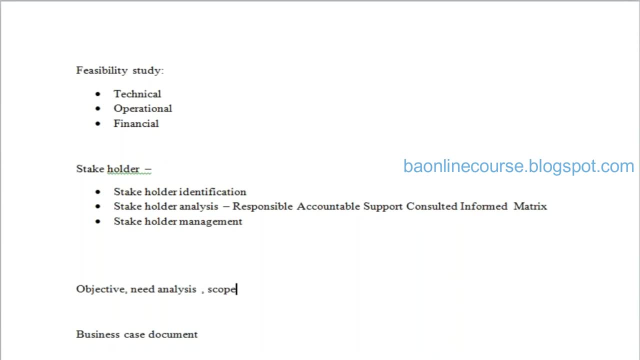 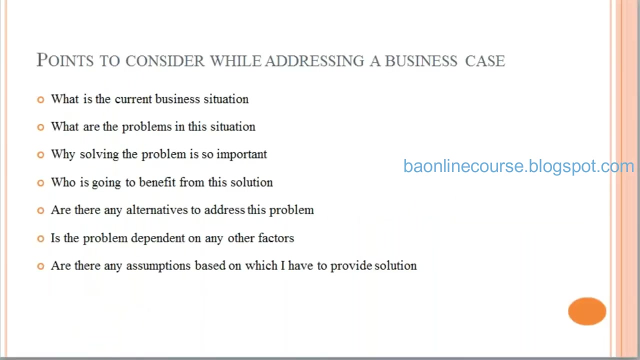 understand. yeah, Emma, yeah, yeah, I'm here, only I'm so. so three points we have to consider. one is about objective. second, we call it as need. third, upon test scope. these three are important for any of the project, right? so these are all comes under the first cleanse, first layer, and 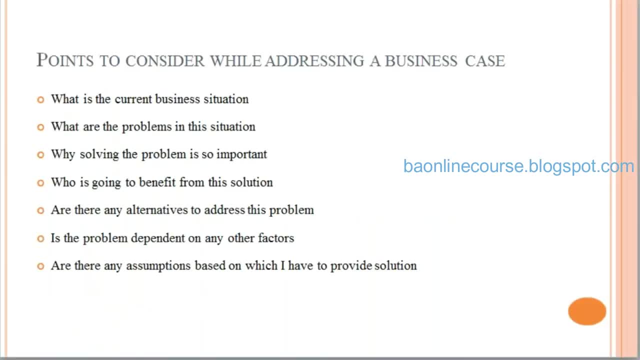 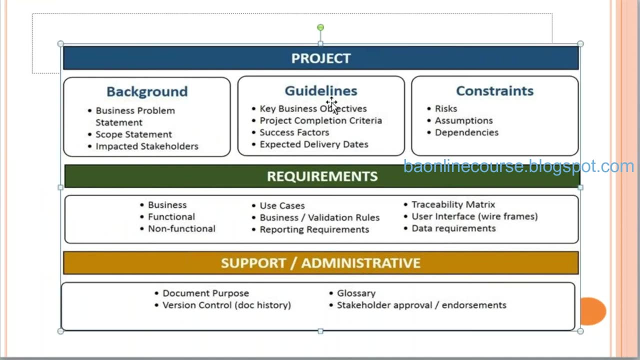 okay, these are all comes under that first layer of the project. so next we call it as guidelines, guidelines and a day. how it is to be done, what are the key business, or in the acumen master. and next you know the completion criteria right at the, a basis on which. 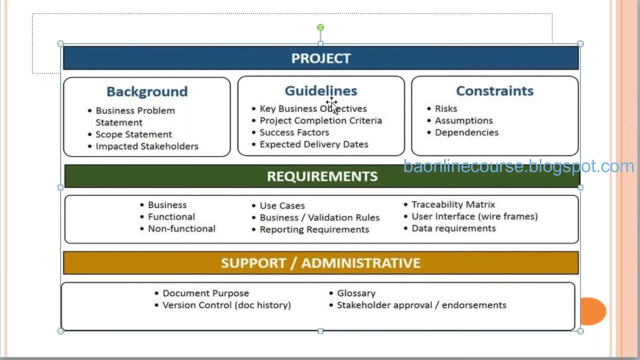 criteria. we have to complete the project and next we have to followed by the success factor, success factors and TNT. what is meant by success factors, the in a CSF and in the critical success factors, and what is meant by critical success factors? what is meant by critical? 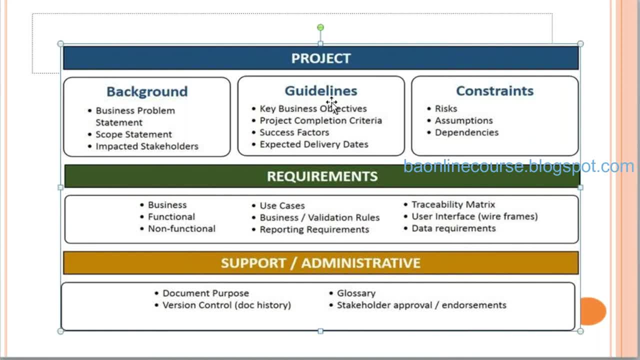 success factor, not surely what is meant by critical success factors, for example? example is done we bother? OK, want to make it successful within the time, what you are expecting in next one year. so this: I want to make it successful. then make so you have the vision. 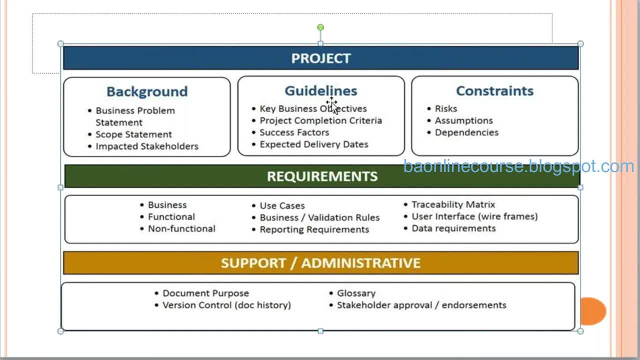 visual income. if you take money, you father says: I buy this new restaurant. so there is a vision. now don't you wonder if you aren't stupid and didn't mean: lugar, come on, huh, to change that ways from one side of you, and that's okay, I'll come to you later, aren't you? 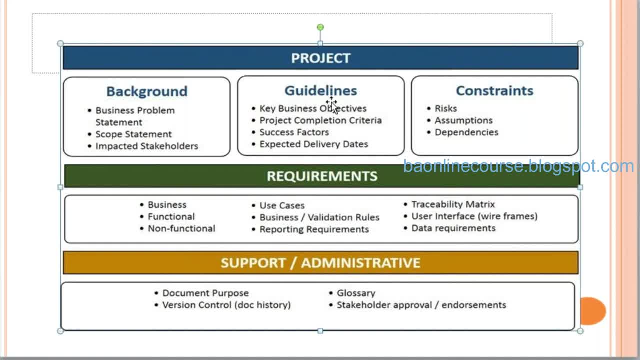 provision on the one year low. success around success: secret inside. that's a secret inside me, it is the new success: a boy, smooth focus. we get a clarity on that. I mean that's it, we're all. the rich are taken on. double on the success of them. I mean I will the parking, the child. he even cover the art in a manum. 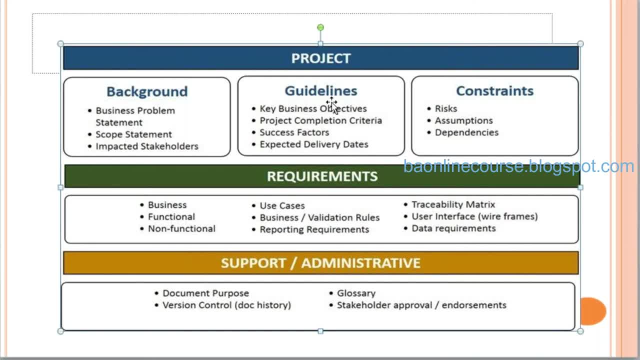 critical success factors and here in Cali for a strength success, ever entry, first and foremost of my children are no logo to to be a student first rating championship chipmunk. she like you know prime location where the location and development a accessibility- yeah, they're a accessibility, the delicious put me reaching it should be. 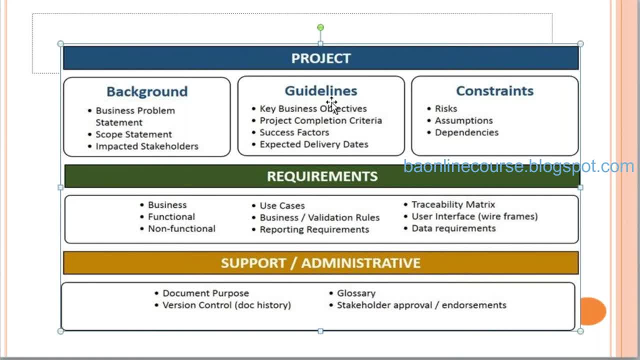 accessible for the public. you know he's an accessibility, but never prime location and right bomb. next, Inca ambience: a munchie cooker, yeah, and beer is Carla. ambience is important you, yeah, and beer is the part in king Ali ambience kiss, supporting a king Ali cook. 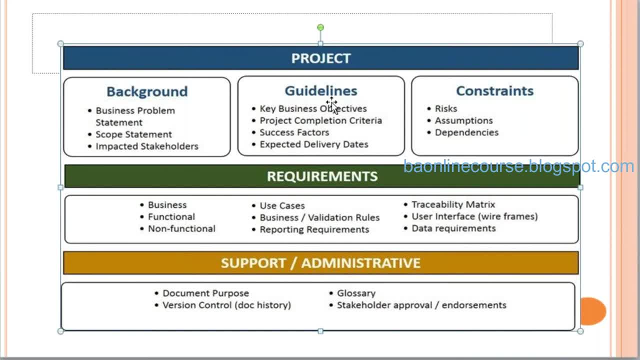 sir munchie, cooks like ambience. expect Jason, or do coding. I expect just ambience. more index suggested what I expect, just a hospitality ambience boundary. I don't know, but it should be hospitality, Calcutta, hospitality and beer. so bodily hospitality, car, delicious food to particle hygienic conditions. 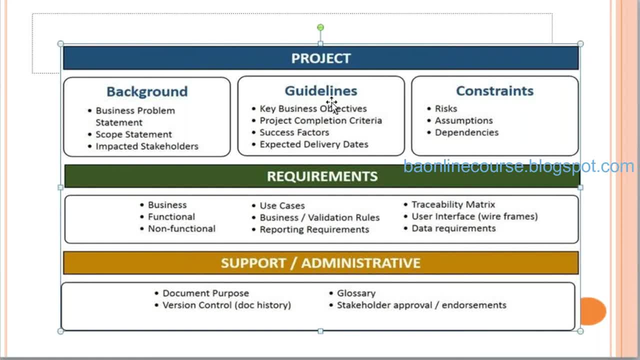 hygiene conditions. you need to kick action. ambience key, hospitality, important. food key, not only delicious, but she really should be. hygiene, the cost-effectively really really add up. okay, just a factor doubt, so we'd mean a real arrow, he won't. a critical success factors. you, even in the store, you should. 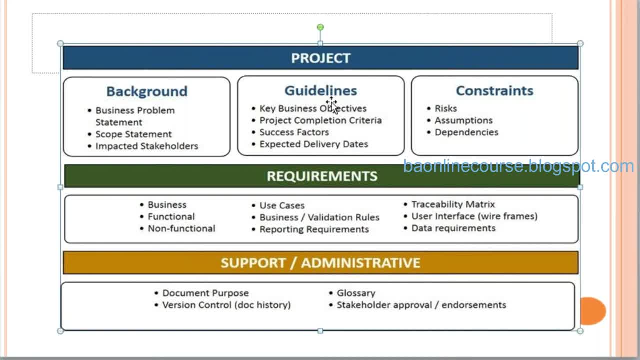 investment. your father told you he is happy. if you don't tell him, he will say: what do you have? what do you have got? simple qualities, what do you understand? it's not only about money. to make your success restaurant successful, there are some factors we have to consider. 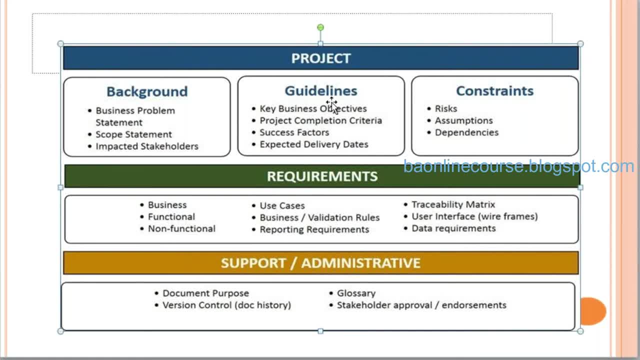 but in the same way, when you are developing the project, critical success factors are also important. when you want to develop any of the project, you have to consider what are the major issues we have to address to make this application successful- not only the solution, but to make the client guard it. 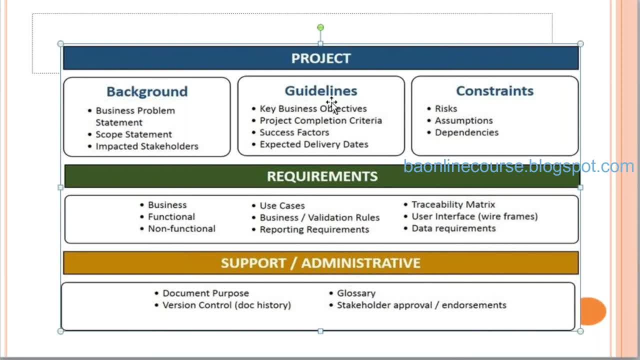 to make it successful, to make it 100% to 300% successful. success doesn't mean you can't complete it. a car manufacturer has manufactured a car. there is no one in the market. there are not even 10 cars in the market. who else appreciates it?